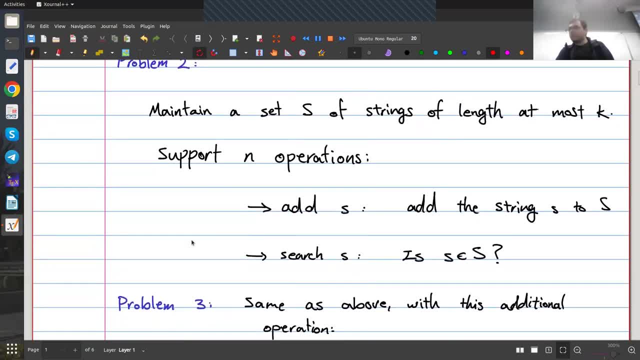 So this is my first problem. The second problem, which is actually, as it turns out, a very similar problem, is that I have a set of strings, Let's say originally, my set of strings is empty, And again, my strings have a length of at most k And I want to do n operations. 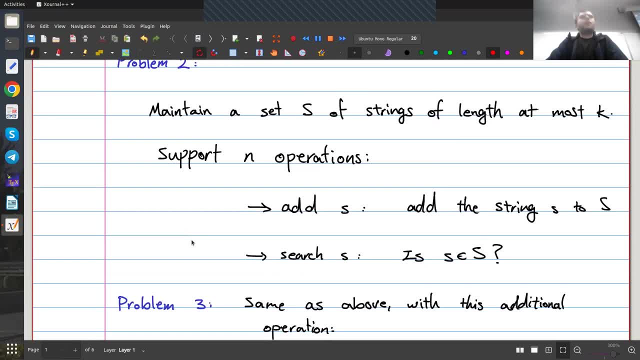 And every operation can either add a new string to the set or it can just ask: is this particular string in the set? So I have an at and a search. This is my second problem. My third problem has the same operations as the second problem. 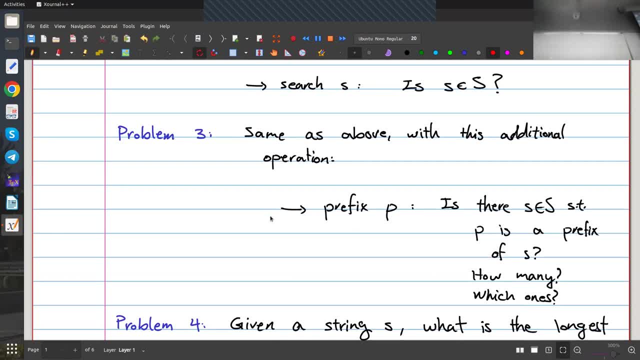 but I have a new type of query which basically gives me some string p and asks me: is p a prefix of one of the strings in your set, Yes or no? And if there is a string in your set such that p is a prefix of it, 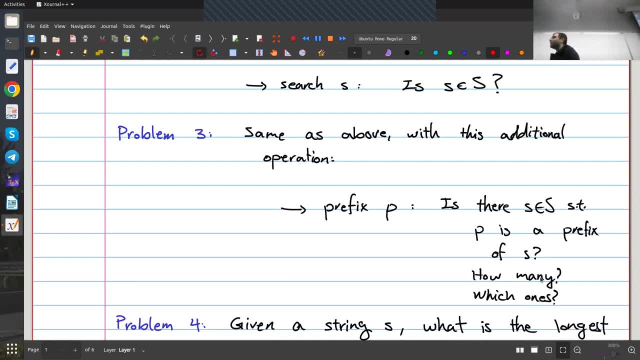 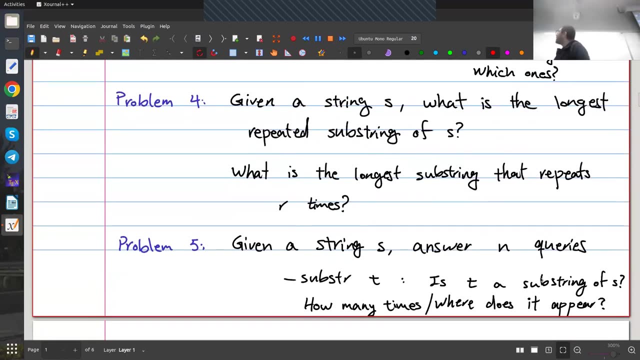 how many such strings are there And which ones are they? So let's say, my strings have indices. I can just output the indices of the strings that have p as a prefix. Okay, So this is my third problem. Now in my fourth problem, 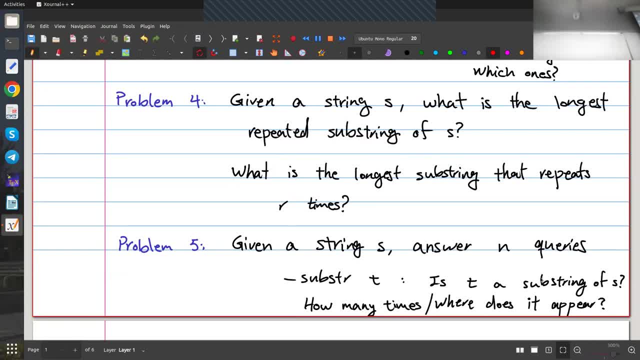 I don't have a set of strings, I just have one string, s. But my question is: what is the longest repeated substring of s? So what is the longest string of s? So I have a string that is a substring of s, starting at two different indices. 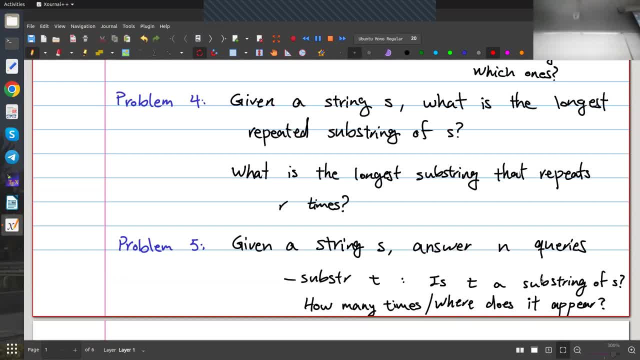 Okay, And I can also generalize this. So suppose that I want to find the longest substring that appears at least r times in s, And again, I'm not talking about sub-sequences here, I'm talking about substrings, So they're going to be contiguous. 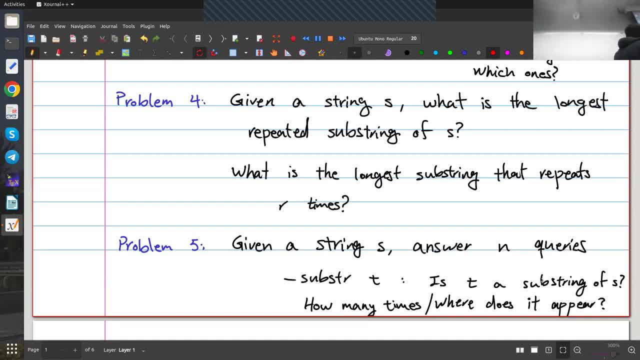 Okay And finally, probably the most important problem. problem five is that I have I have one string s in the input and then I have to answer n queries And every query just gives me another string, t, And the question is: is t a substring of s? 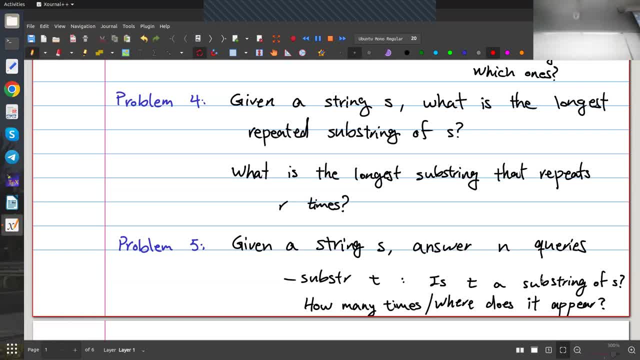 And again I can generalize this. I can ask: if t is a substring of s, then tell me how many times it appears in s And also tell me where in s it appears. So give me all the starting indices, such that if I start there in s. 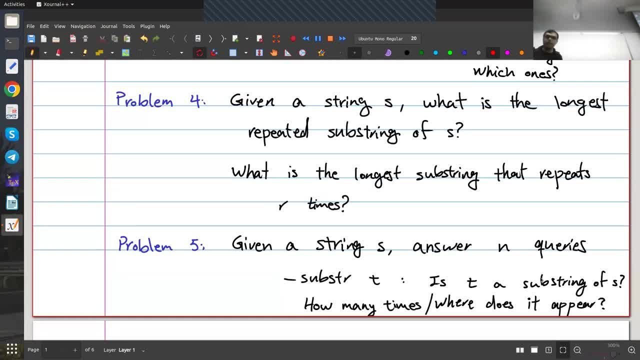 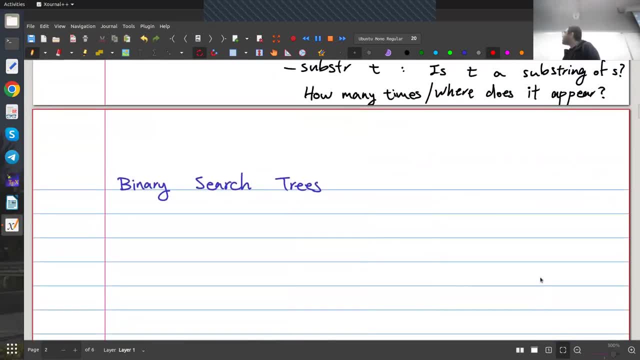 I would see. I would see a copy of t. Okay, These are the problems we want to answer. Well, we saw basic sorting, but we can also use binary search trees, right? So let's say, I just keep a binary search tree of all of my strings. 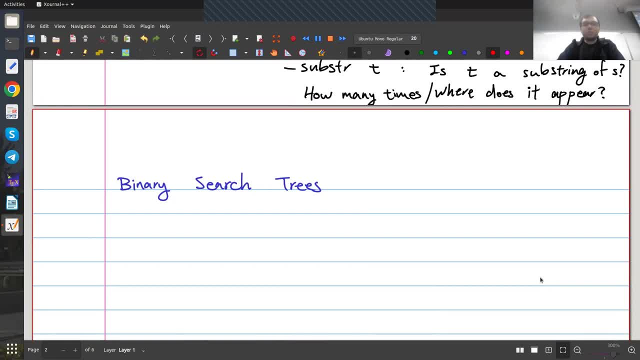 And whenever I want to insert a string I just do it. So let's say it's also a balanced binary search tree, So it's an AVL tree or any other kind of- I don't know- balancing, And so the height of my tree is all log n. 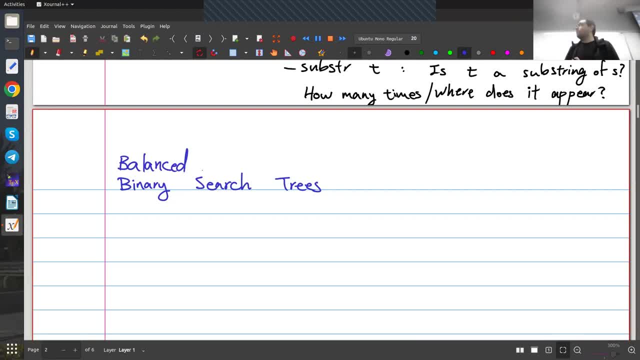 And at every node of my tree I'm saving a string. And basically, when I was teaching you binary search trees, I said that the only thing we need is some process to be able to compare two of the items. And I can compare two strings. 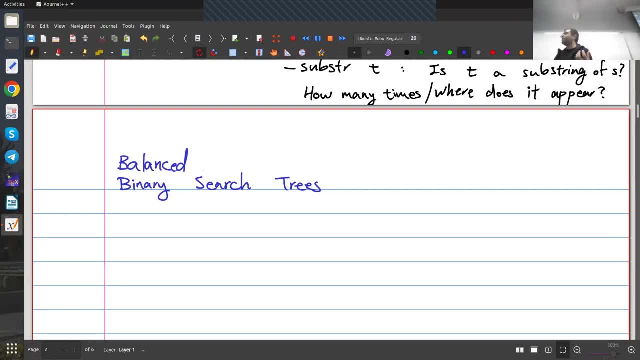 right. So it makes sense to say that this string is smaller than another string. It just means that it's it comes first alphabetically, right, Or comes before that one alphabetically, and so on. So I can just create a binary search tree. 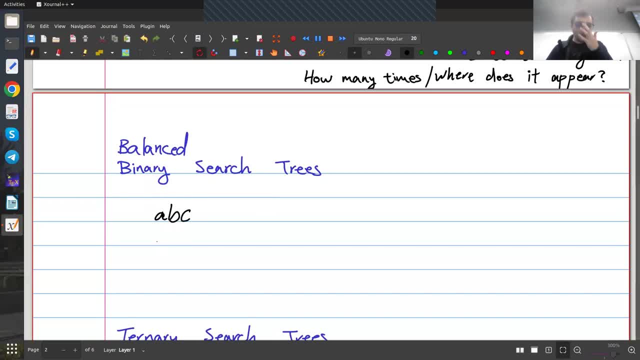 For example, if my strings are ABC, ACD, BCE, I can just create a binary search tree. I put ABC here and then ACD is bigger than ABC. So it goes to the right, and BCE is bigger than ABC, And it's also. 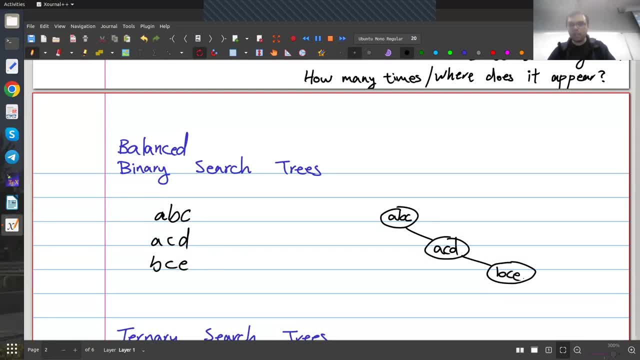 bigger than ACD, So this one also goes to the right. So this is just a binary search tree. I just have strings. Now, of course, this is not balanced. I could also have the AVL version of this so that I get everything balanced. 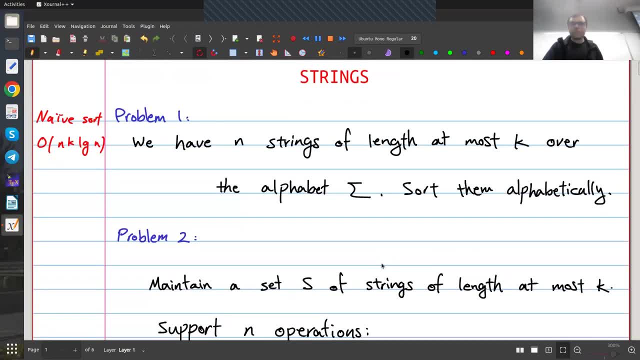 Now what happens if I use a balanced binary search tree? which one of these problems can I solve? Well, I can solve this first problem by just inserting all of my strings into the tree and then printing them in order. right, But this one would give me the same runtime. 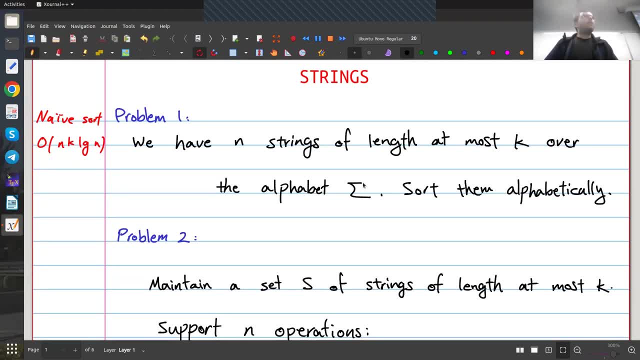 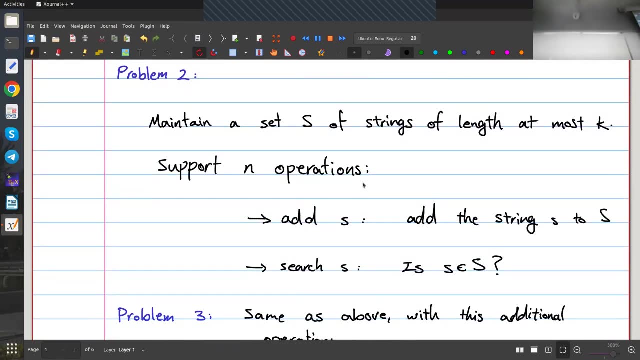 as the naive sort, Because again I have n log, n comparison operations in my binary search tree and each comparison is now taking okay time. So the runtime is still NK log. What about here? Well, I have a set of strings. 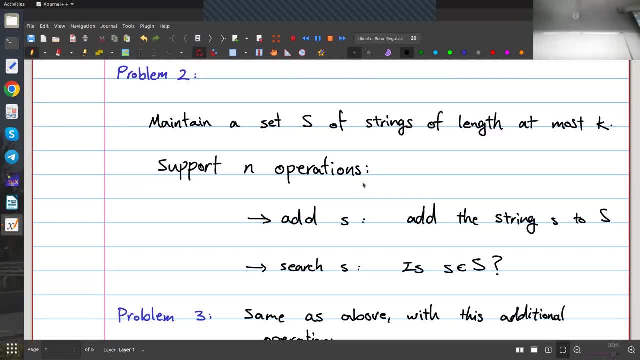 I have n operations, so I have at most n strings in my set. Whenever I'm adding again I need log n comparisons to add in a balanced binary search tree or log n comparisons. but now every comparison is taking okay, So every add takes okay, log n. 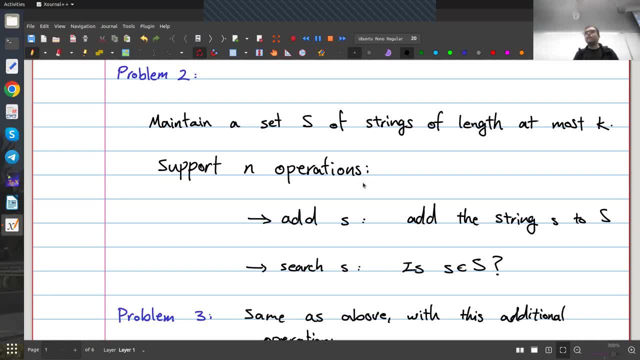 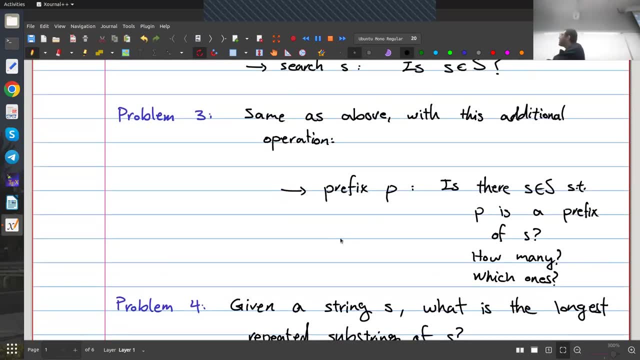 and every search also takes okay log n. Okay, Now how about this one? If I have a binary search tree of my strings and then I find some string that is a prefix of p, can I figure out what is the number of strings? 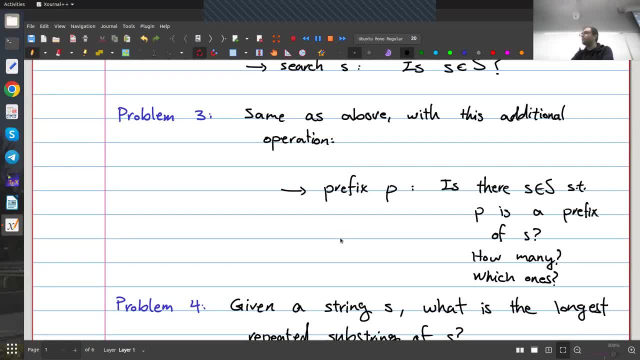 such that p is a prefix of them. Can I like count that or find them just based on the ordering in my binary search tree? So the thing that you have to realize here is that if p is a prefix of s, then p comes before s in the object. 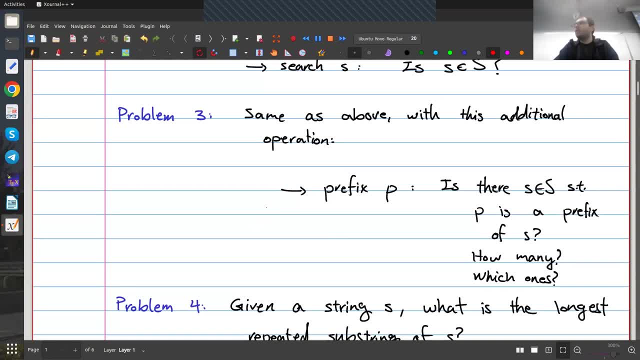 So if p is a prefix of s, then p comes before s in the object In the alphabetical order, right? So if I have all of my strings in a binary search tree and I'm asking: is there a string s that has p as a prefix? 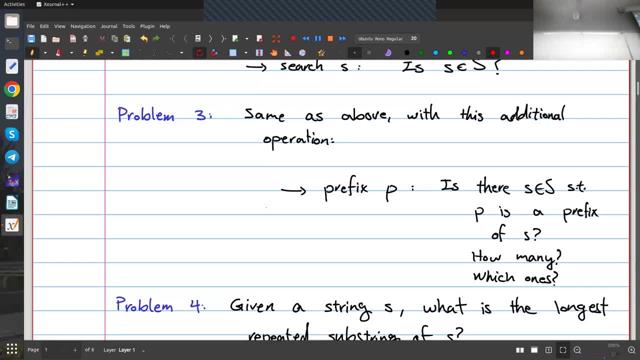 then this s should definitely come after p in my order, right? But now I can have, let's say, I just invent a new letter and add it to my alphabet, And let's say that this letter comes after all of the other letters that I had in my alphabet. 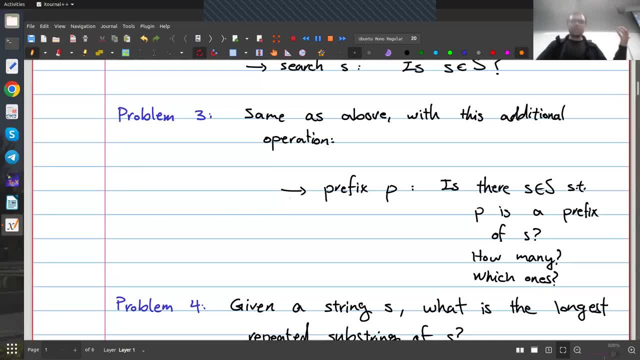 Okay, let's call this letter, let's say alpha. Suppose I'm using the Latin alphabet and I'm suddenly adding a Greek letter in there. Okay, so then if P is a prefix of S, then S would be bigger than P. 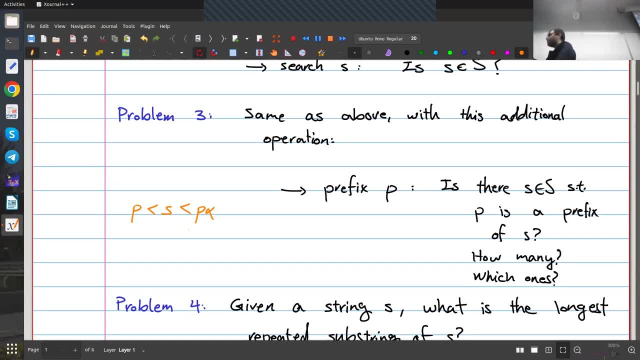 but it would be less than P alpha. This is the string P with the character alpha added to the end of it, right? So actually, if I want to see how many strings S have P as a prefix, I'm basically asking how many strings S. 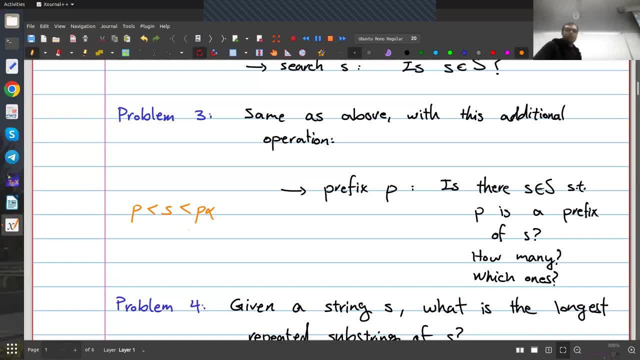 are between P and P alpha. So this is two rank queries on my binary search tree. And again it takes all K log N, because each one of them takes K log N. And again the comparison, every comparison, is taken, So I can answer this in K log N. 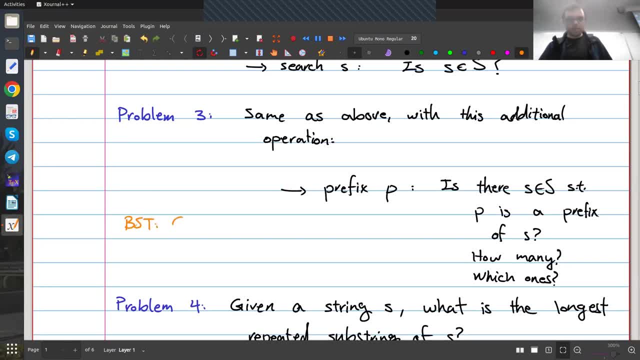 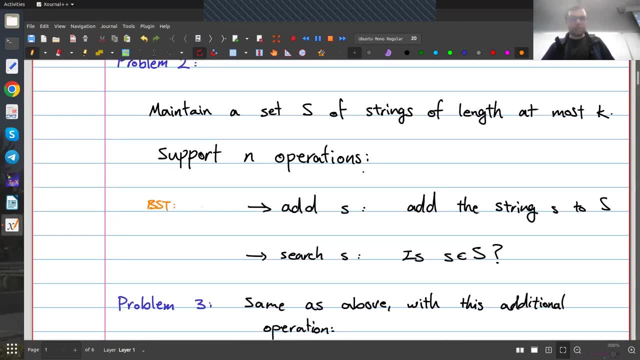 That's. Let me write it somewhere. So it's binary search tree. This is K log N And these ones are also K log N with the binary search tree. Of course, we want to do better than this, if we can. 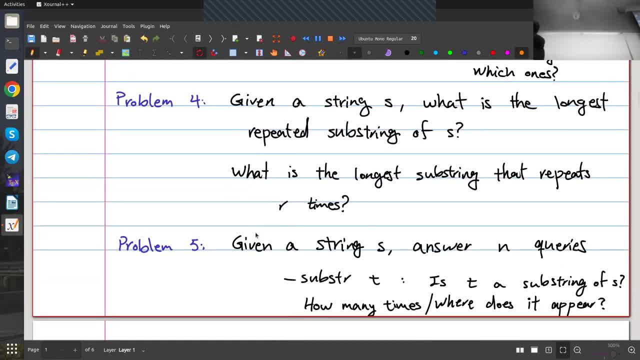 Okay, how about this one? Given a string S, what is the longest substring of S? And here let's say that the length of S is K. I'm generally using K in this lecture for the length of the strings. Okay. 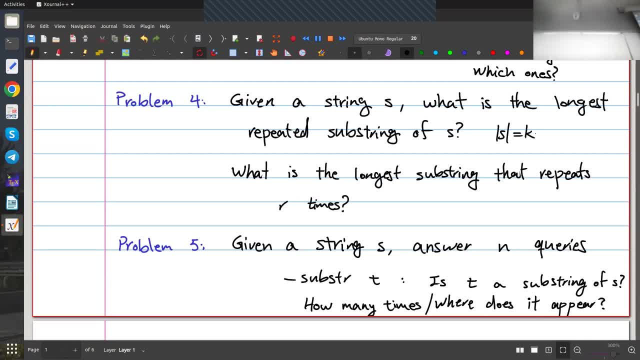 So I can just create a binary search tree in which I add all of the substrings of S. Right There are N squared substrings of S, So if I add all of them into a binary search tree, the total runtime would be N squared log N times: K. 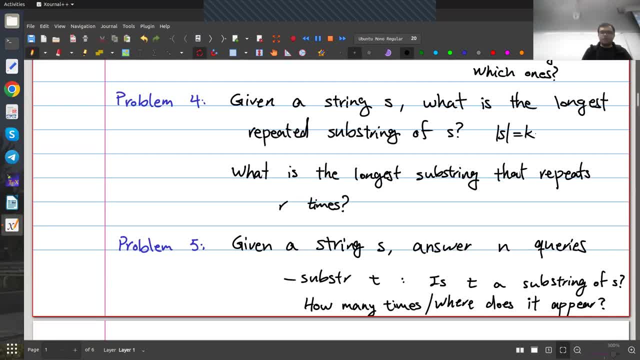 I always have the times K for the comparisons, right. So that's my pre-processing. And then whenever someone gives me a string, I just have to check: is this string in this binary search tree? And that's all. K log N. 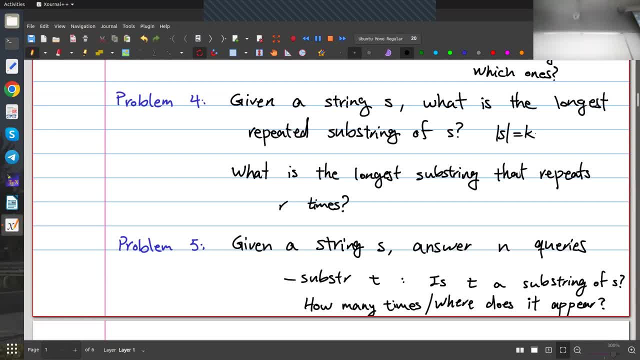 And also I can just count how many times every substring appears and so on. So this part is also fine, But again really slow, And yeah, So I can figure out if it repeats. I can also answer problem five like this: 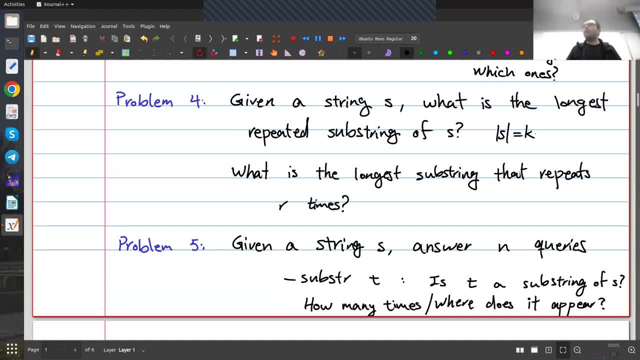 Both of them, as long as I just keep a set of all the substrings Right. But of course, the whole point of this lecture is that this is wasteful and it's going to take too much memory and also too much runtime. 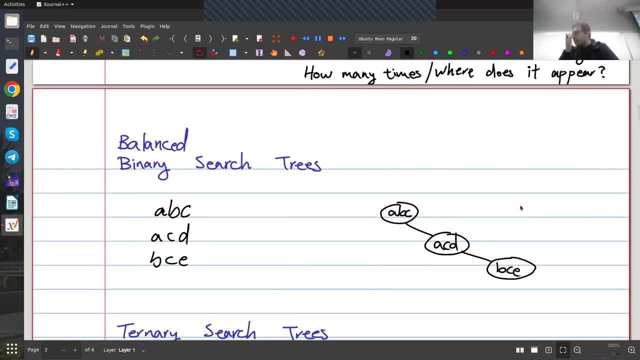 So we want to do something better. Now, the first thing I would mention here is that I really hate the fact that I had this K appearing in my runtime, Because every time that I was comparing, I had to compare two whole strings, and that took okay time. 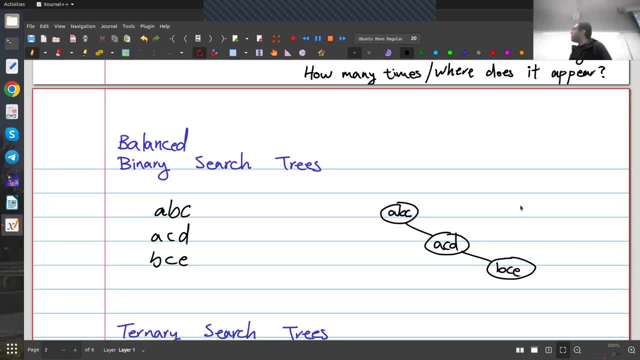 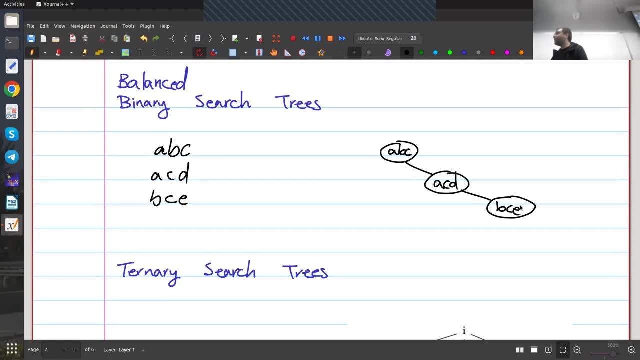 So all of my runtimes were multiplied by K. So I'm going to have a different data structure and we call this a ternary search tree, And the idea is very similar to a binary search tree. I always want to compare and, based on the comparison, decide whether I go left. 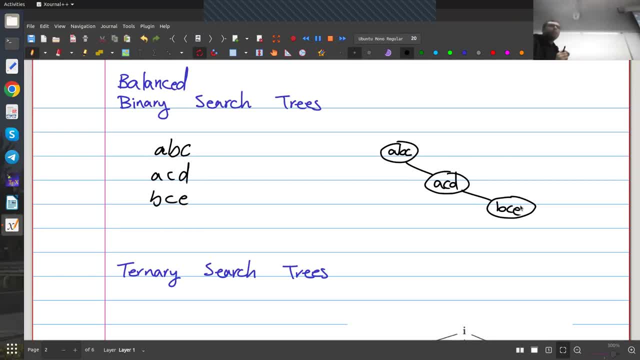 or right or so on. But I want to make sure that my comparisons are always on just one character. I don't want to compare whole strings, I just want to compare one character of this string with one character of that string So that I can say all of my comparisons are done in constant time in all one. 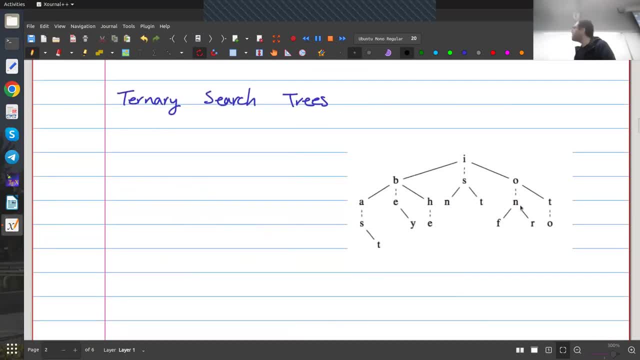 Okay, Now, how can I do this? Well, here's an example of a ternary search. So I start at the root and I have one character at the root, In this case I. So let me just tell you how I search for a string here. 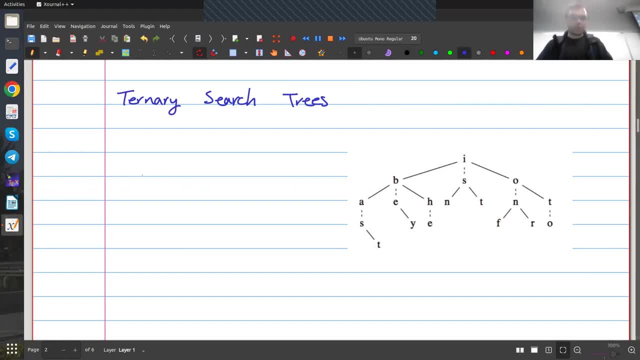 Suppose I want to search for a string. For example, I want to search for at: Okay, I think the first character should be A, But the first character at this root is I. So I'm looking for a string that has a first character smaller than I, because A is smaller. 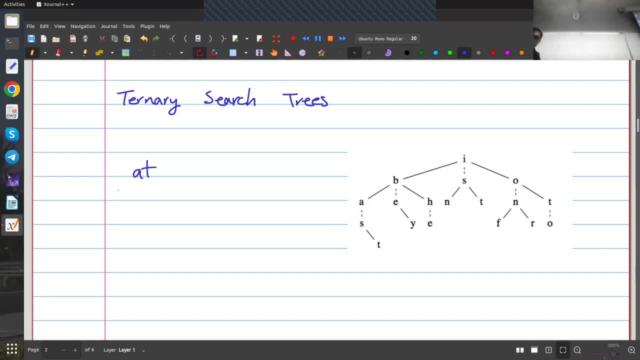 So I just go to the left child. Okay, Now, this left child, This B, corresponds to the strings whose first character is B. Okay, But my first character is A, So I need a smaller first character. I'm going to again go to the left. 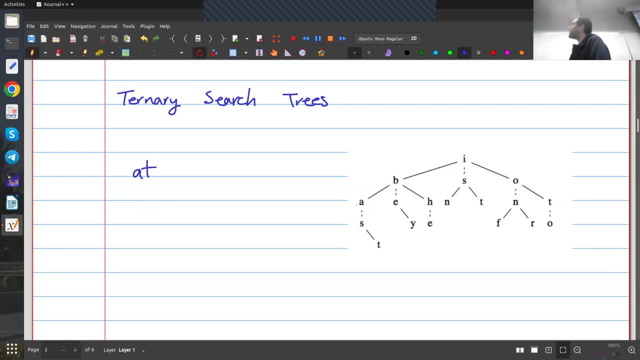 So now this A corresponds to all the strings whose first character is A. I'm happy with this because my first character is A, So as soon as I matched my first character, I go to the second character. So now, Remember, this is all the strings whose first character is A. 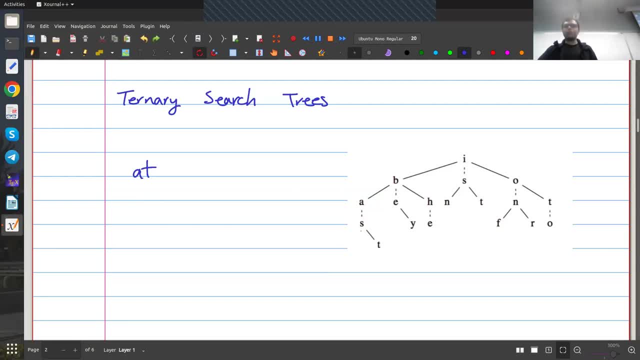 Now I'm going to the second character. This one corresponds to the strings, whose second character is S, But my second character is T. T is bigger than S, So I'm going to go to the right And so on. So, generally speaking, 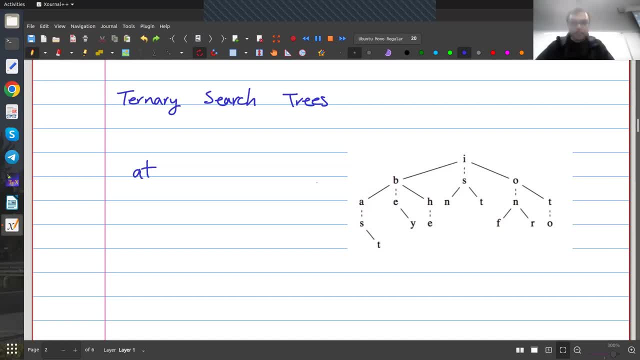 The way this works Is that Let's say I have indices, So let's say I'm going to start with index zero or whatever. So my index zero is A, my index one is t, so the root always corresponds to index zero. okay, and i have some character there. 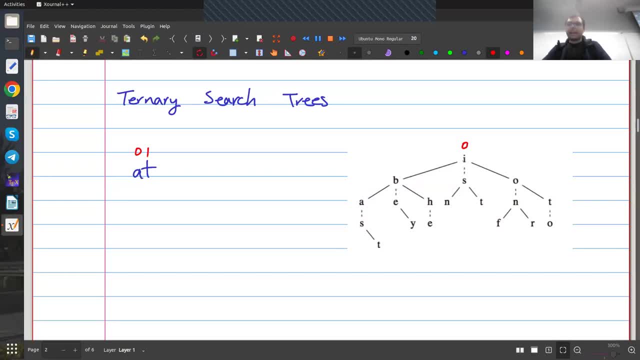 so all the strings that have their character at index 0 smaller than this root would be to the left. all the strings that have their first character character 0 larger than the root would be to the right. but then in this case we have an equality as well. right, so i might have. 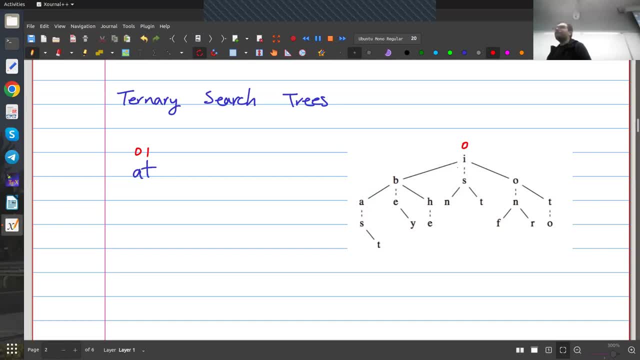 some strings whose first character is exactly i. that's why i have a ternary tree. every node has three children. so these are the strings whose first character is less than i. the root, these are the strings whose first character is larger than i. and now these ones are the strings whose 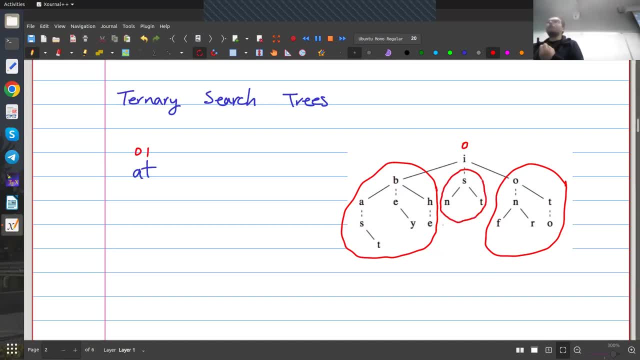 first character is i. but as soon as i know what the first character is, i'm going to focus on the second character. so now the roots here in this subtree. s it corresponds to all the strings whose second character is s okay. so in general, every node has three children. it has a left child. 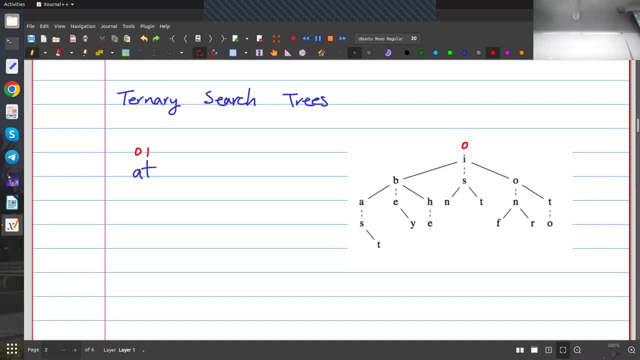 a right child and a middle child or an equality child. okay, and the idea is that if this node is talking about some index, for example, this node is about index zero- then its left child and right child will be about the same index, but its middle child would be about the next index. okay, so again, this b it corresponds to: 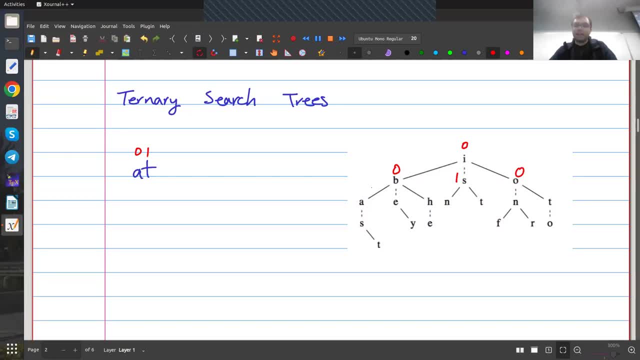 all the strings whose character at index 0 is b. so its left child will also talk about strings whose character at index 0 is a, and this is also at index 0, but its middle child is at index 1.. so you can continue like this. so this s is actually at index. 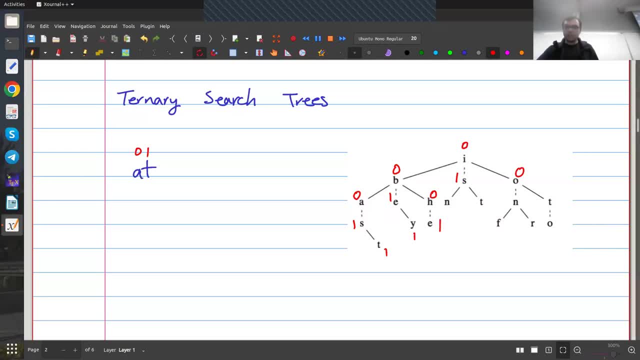 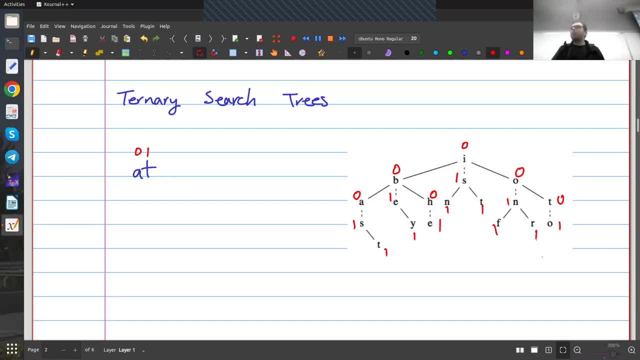 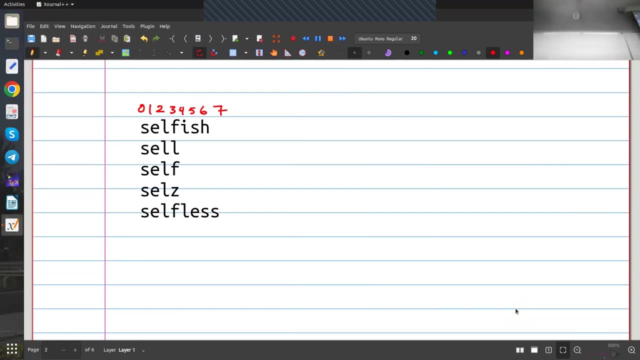 you're going to the next character, to the next index, but whenever you're taking the left child or the right child, you're doing exactly what you were doing in a binary search tree. that's the idea of a ternary search tree. okay, let's create a ternary search tree on these words. so i want to show you how to insert in a ternary 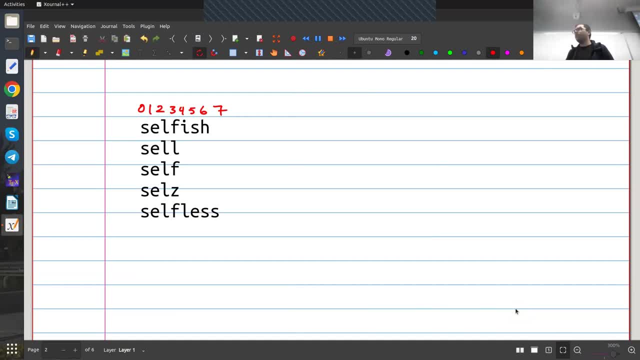 search tree and then i want to show you how to delete and how to search. okay, so first i start with an empty ternary search tree and i want to add the word selfish, so i add s now. at this point i don't know any of these future words. okay, so i only know the word selfish at this point. 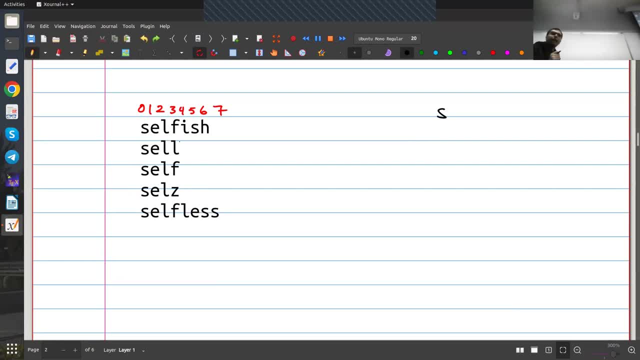 so when i add s, all of my words have s as their first character. so i don't need a left child or a right child, i only need a middle child. so i add a middle child, and we said that whenever we have a middle child, we go to the next character, which is e in this. 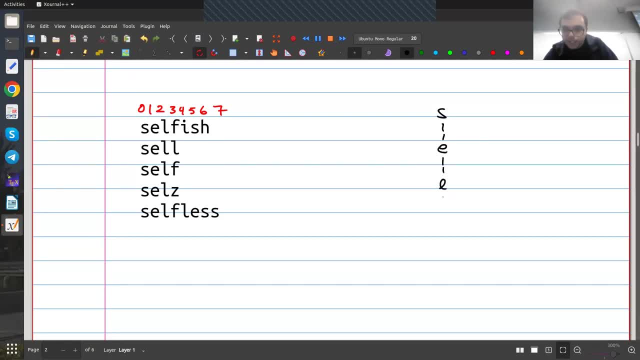 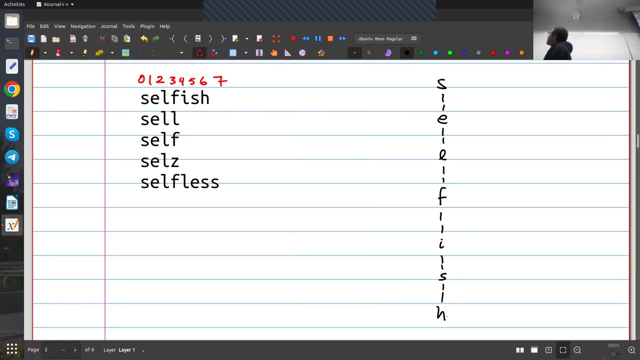 case and basically i continue like that. so my first insertion is always like this: ah, it didn't fit, okay, so this is selfish. now i want to add my second cell. now i compared the first character. i see that it's s because it matches. i can now go to the. 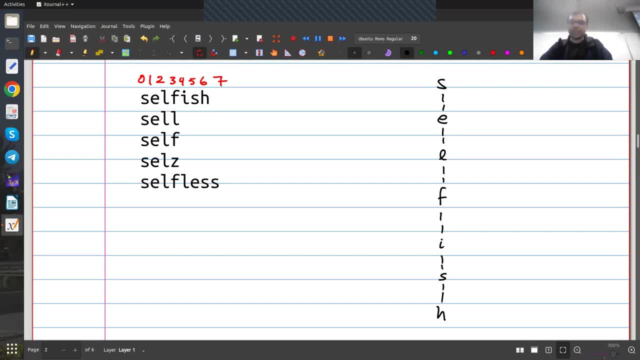 second character. so i take the middle child and go to the second character. it's e. this one also matches. so i take the middle child and go to the third character: it's l. this one also matches, matches. I take the middle child and go to the next character. Now in the tree I have f, but in 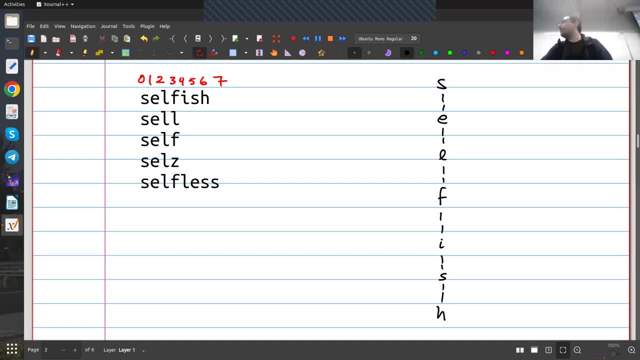 my word. I have an n, So l is bigger than f. so this should become the right child of f. So this is how I add the word send. Okay again. so this is the first character. this is the second. third, this is the fourth character, but then I'm increasing the fourth character to l. basically, that's how you. 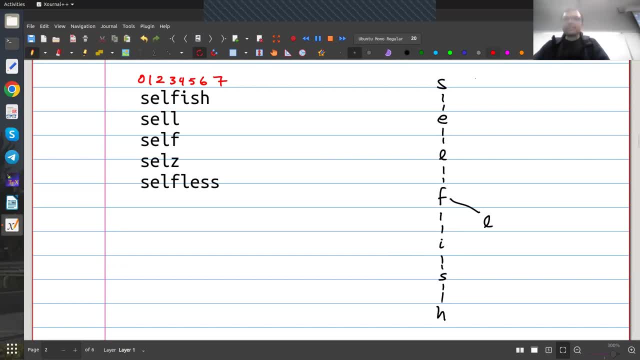 have to see it. Okay. and also, let's say that at every node of my tree I keep a boolean to know whether I have a word here or not, because, for example, I don't have the word se right. So I want to have a boolean, let's say a check mark, saying that the selfish was a word and this cell was also. 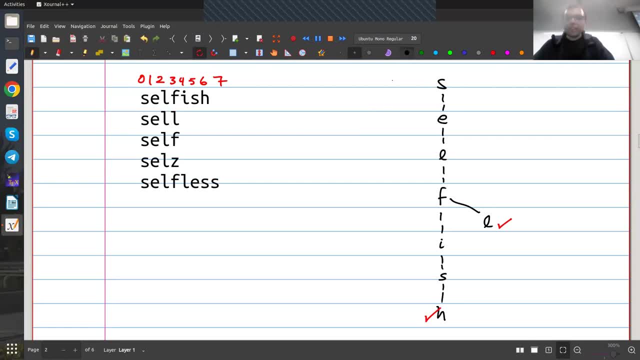 a word. Now I want to add self Again. I start here. s is fine. it matches the first character. so I go down the middle E matches the second character. I go down the middle L matches the third character. I go down the middle F matches the. 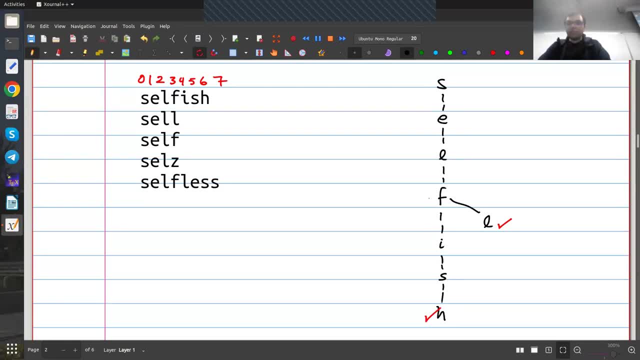 fourth character. so I have a perfect match. I didn't have to add any new nodes. I just have to remember that this is the end point of a word. Okay, now let's say so many words, what is this? so I go s, e, l, and now I go to f, and I see that it doesn't match because I need a z, so z is bigger than. 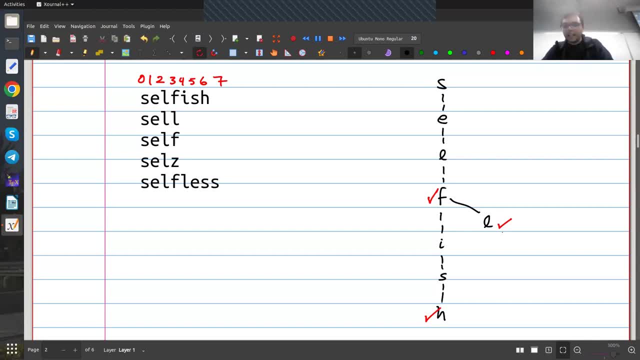 f. now I do what I did in a binary search tree. I go to the right, I see an l, but z is even bigger than an n. so I would just again create a right child and add z here, and I put a check mark to remember that this is the end point of a word. and finally I have selfless. so I just go down here, self, and 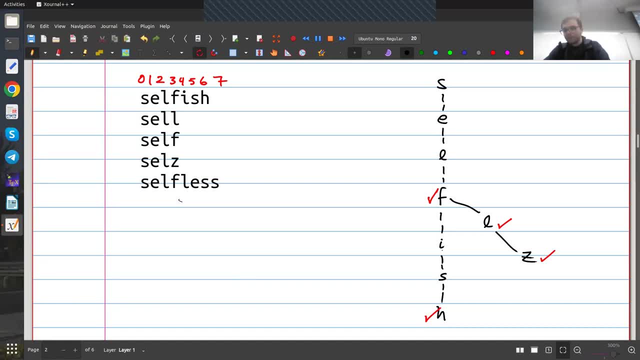 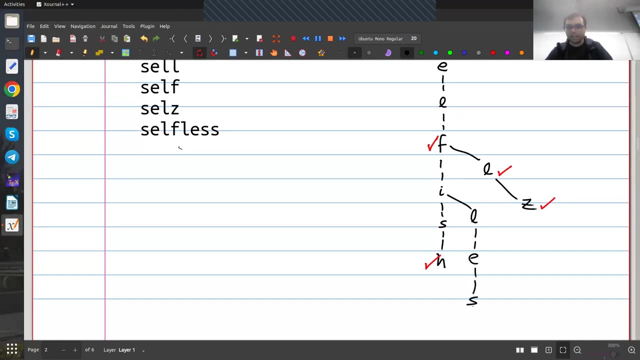 then I go down one more time, I see that I have an i, but I need an l. l is bigger than i, so I will create a right child l, and then the rest of this is just as before. it's e s s. so this is how I would. 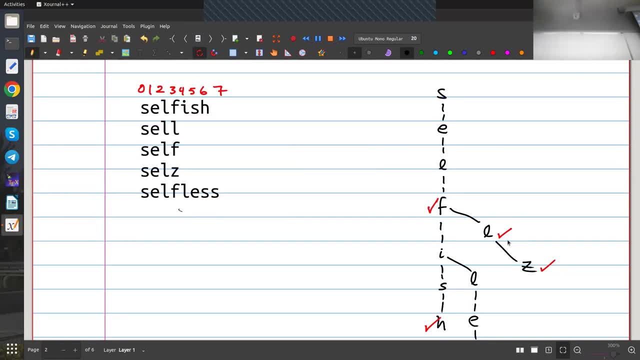 insert. now, how would you search? well, when you search, you just do the same thing: just go down your tree every time. if you don't have a match with your current character, you have to go either left or right, depending on how you compare, and if you do have a match, you just go down the middle and then you go. 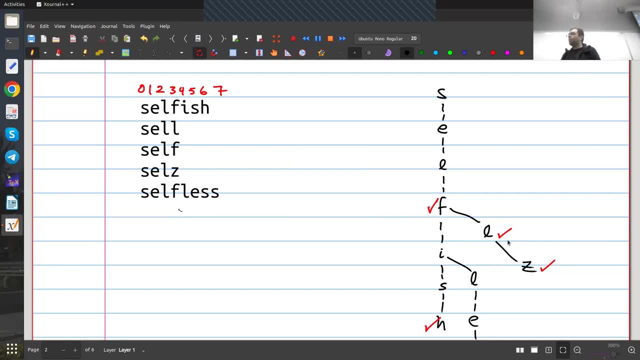 to the next character. start matching the next character. okay, what is our runtime? so, for example, what is the runtime for a search here? let's say that I have added all of my n words and let's say that each of my words has, at most, k characters. okay, 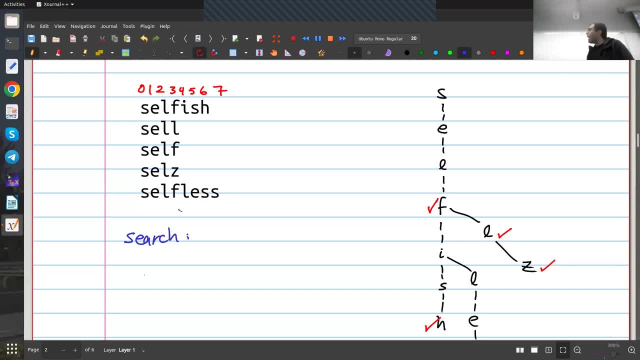 and now I'm searching for a particular word. and let's say the height of this tree is h. okay, so you have to decide on two things: how many times would you go left or right? right, so the number of times that you go either left or right is basically, at most. 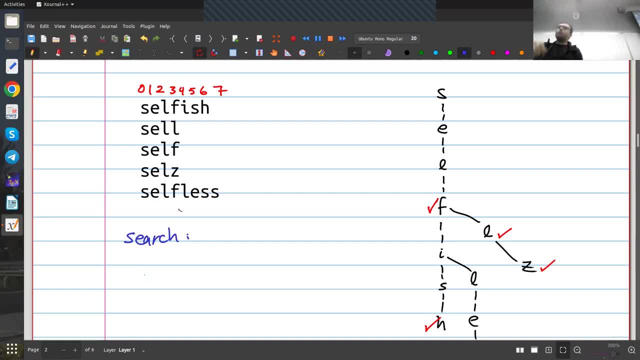 the height of the tree and how many times will you go down the middle? at most k times, because every time that you're going down the middle you're matching one character. so the total runtime for search is actually all k plus h, where k is the length of the string that 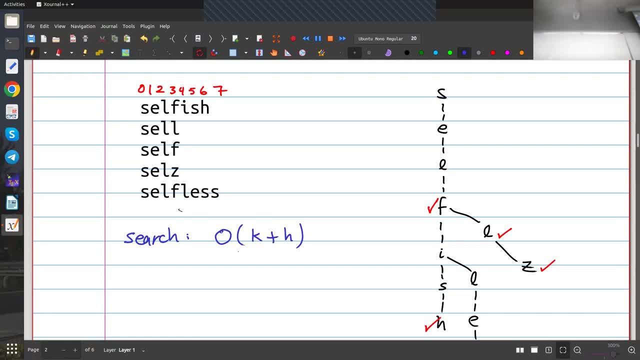 you're searching for and h is the height of your tree. okay, but then you can see that all of the other operations take the same time as well. so if I want to do an insert, it's basically the same. it's k plus h. if I want to remove something, by the way, removing is super easy, just search for it and. 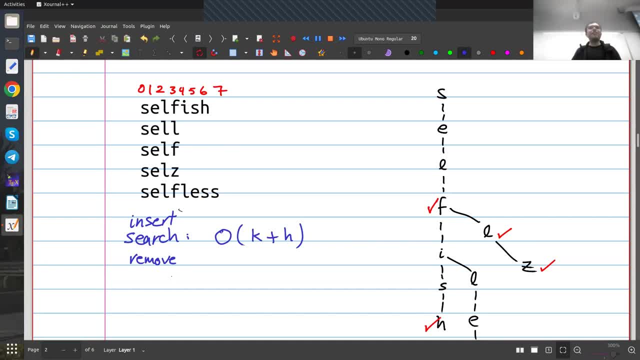 remove the checkmark. right, you don't even have to to hear the vertices that you don't need, just remove the check mark, okay. so everything is done in runtime, all k plus h. so we are in a situation very similar to binary search trees. if I have a balanced ternary search tree where this h is log n. 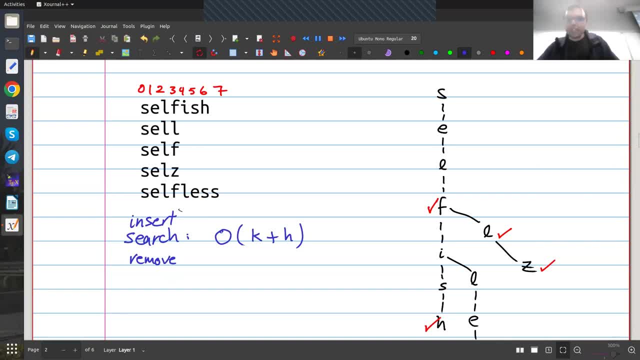 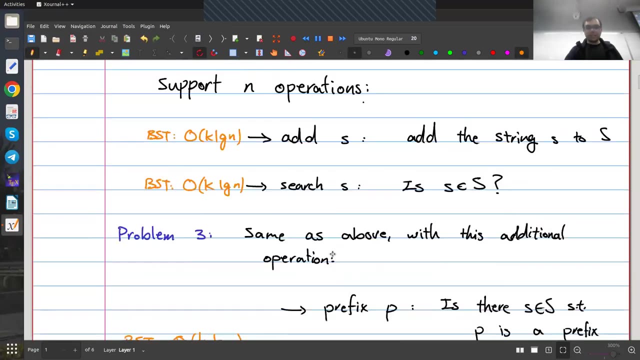 then each one of these operations would just take all the values of this tree and then I could just o k plus log n. okay, if it's balanced, if the height is o, log n. And this is much better than what we had with the binary search tree, because in a binary search tree each operation took k. 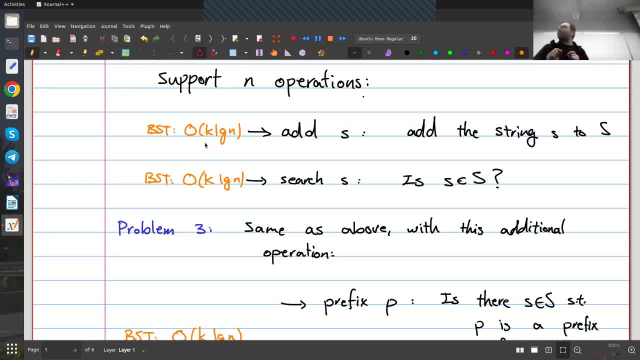 times log n, but now I'm spending only k plus log n. k plus log n is much better than k times log n, of course. So in a ternary search tree, this is not the famous TST, it's k plus log n. 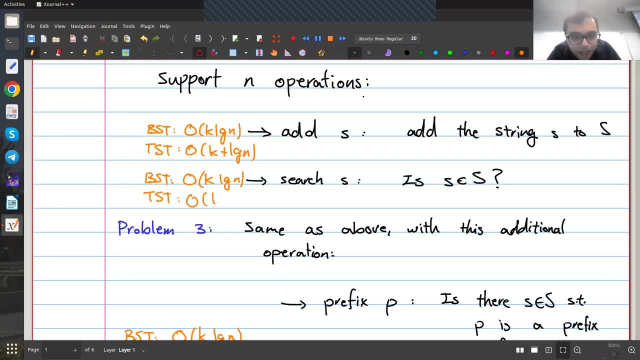 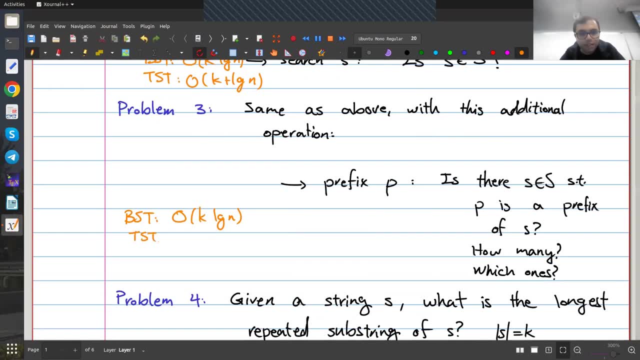 And this is also k plus log n. And this one is also k plus log n, because you can actually do the rank operations as well. Everything is very similar to binary search trees, except that you have to always remember that if there is equality, I just go to the next one. 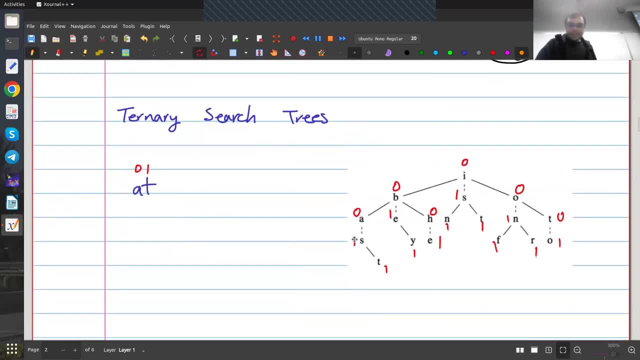 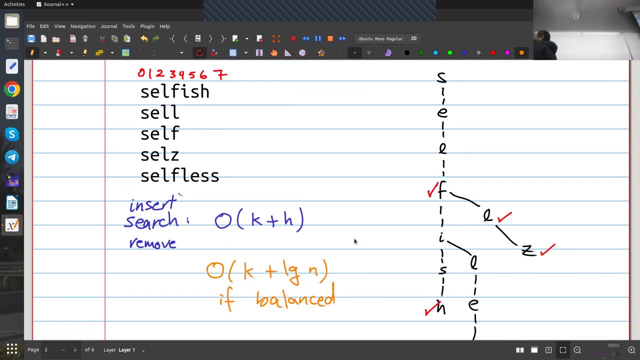 Next character. Okay, But this is assuming that we have a balanced ternary search tree, and what I showed you was just a normal ternary search tree with no balancing. It turns out you can do rotations on ternary search trees as well. 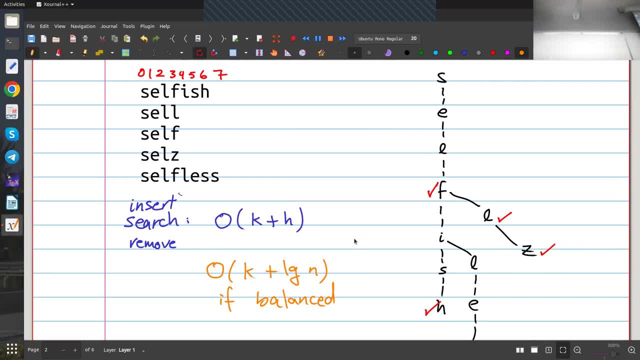 So you can have, like the ternary variant of ABL trees. Now, I'm not going to teach that The rotations are actually very similar to ABL rotations, but all you need to know is that we can make this tree have a height of log n, and then all of these things will work in k plus. 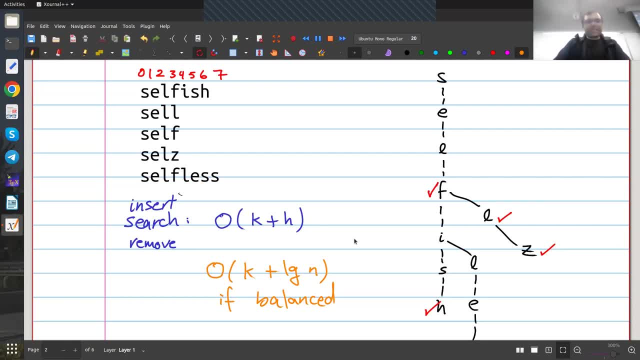 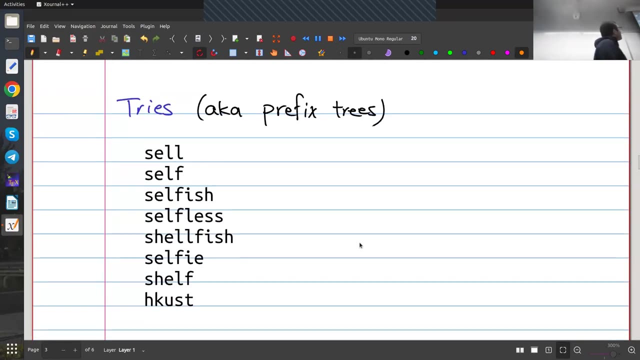 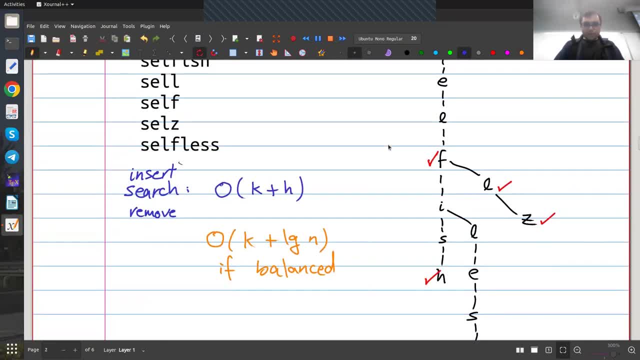 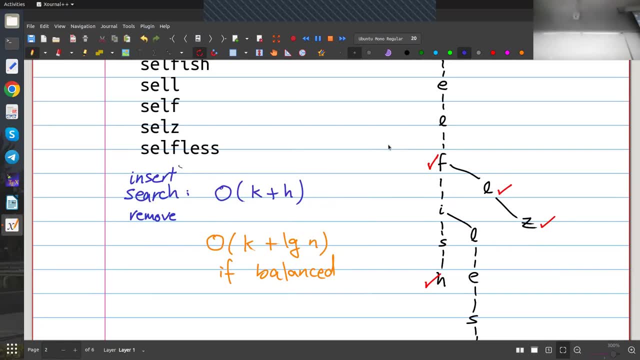 way of saving strings. Okay, But before we do that, I just want to say one thing here. What is the main operation that I'm doing in my ternary search tree? It's comparison, but it's comparison in big characters, So I'm not assuming that my alphabet. 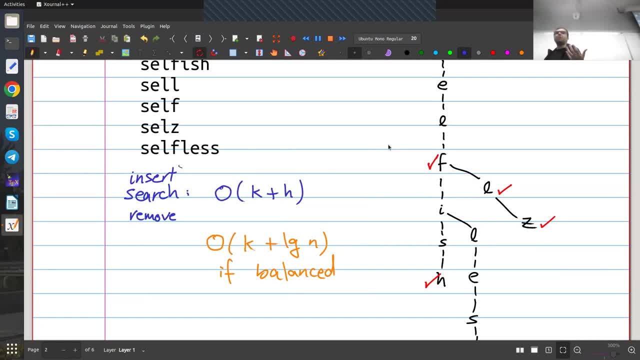 is small, I can have a huge alphabet here. For example, my alphabet can just be, let's say, 32-bit integers or 64-bit integers. As long as I can compare two letters in my alphabet, I can use this. So I can use this to sort also, let's say, vectors of integers instead of just. 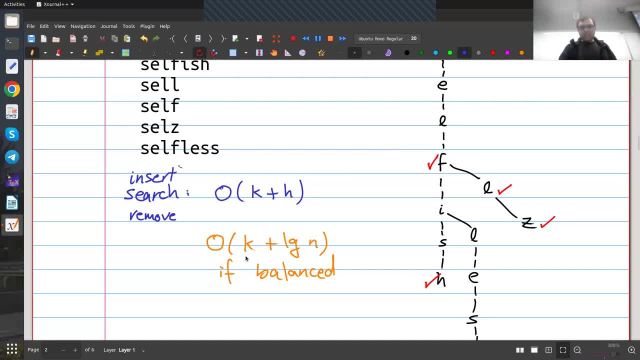 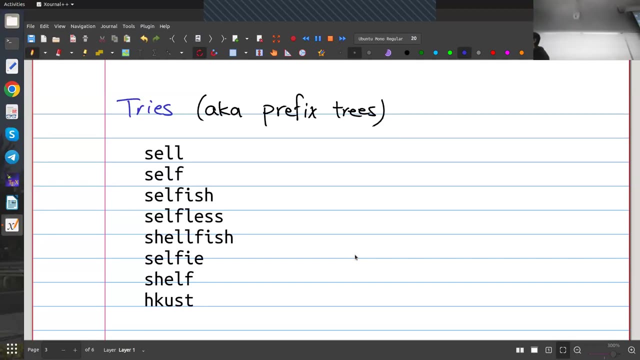 strings. And the good thing here is that I don't really care about the size of my alphabet as long as I can compare two letters of my alphabet in constant time- And I never compare two complete strings. But now, from this point onwards, I'm going to assume that my alphabet is small, Okay. 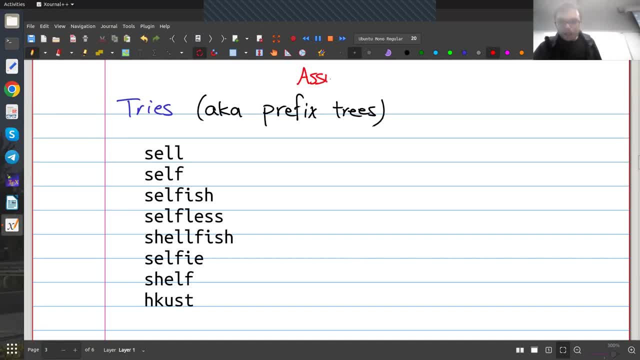 So in the previous one I wasn't assuming this, But from here onwards I'm assuming that the size of my alphabet is small, And this is actually one of the reasons why I'm going to get better run times for all of my algorithms. And this is fine if you're working with, let's say, binary strings. They're just 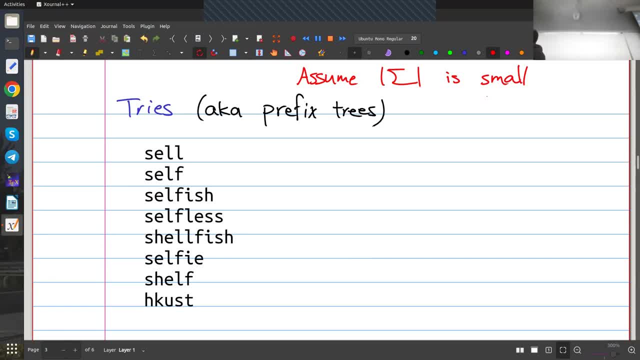 zero or one, Or if you're working with strings that are written in English and you have 26 letters, Or actually. the main use case is in computational biology and bioengineering, Because I have a lot of experience with bioinformatics, where they're processing DNA. 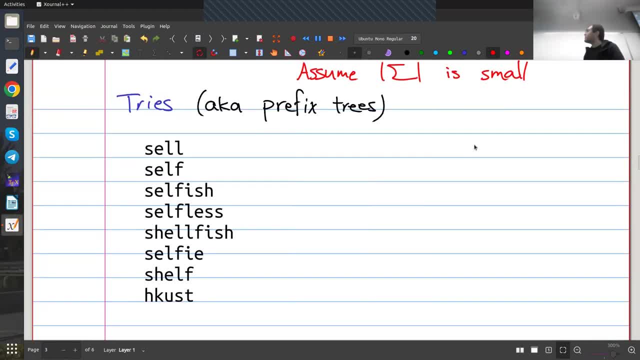 and they have four letters. So let's talk about tries. What are tries? Or also sometimes called prefix trees. So basically, the idea is that I'm going to save all of these strings, But I'm going to save the strings one character at a time. So, for example, when I want to save the 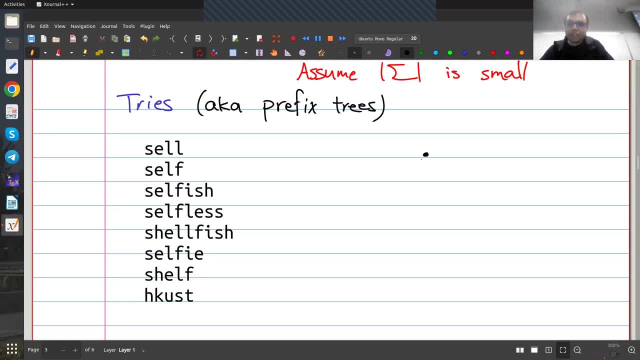 string cell. I'm just going to do this. I'm going to create a vertex. It's going to have an edge that is labeled S. By the way, I'm labeling my edges. now You can also label the vertices, It doesn't really matter. And then I create another edge called E, And then 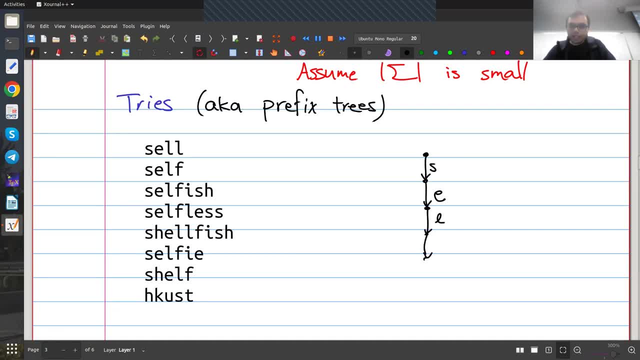 another edge labeled L, And then another edge labeled L. So this is how I want to save one word. But now, the next time, when I want to save the next word, I reuse what I already have. So I start at the same rule. 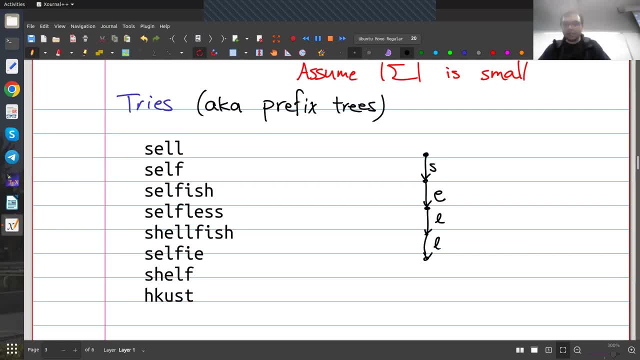 So this root corresponds to the empty string. This vertex corresponds to the string S. This vertex corresponds to the string SE. Every vertex basically corresponds to the string that is obtained if you start at the root and go all the way to that vertex. So now, if I want S, E, L, F, I already have S, E and L here. I can just add a new vertex here for F. 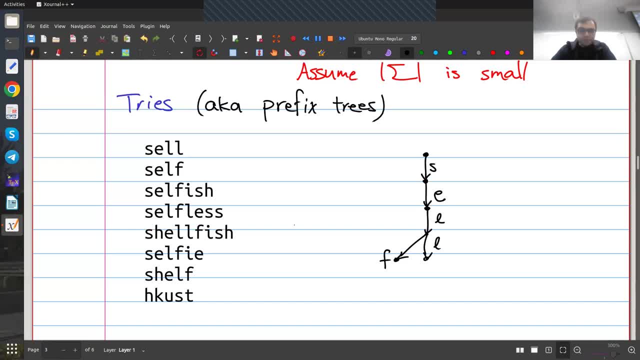 Okay, Now if I want to have selfish, I do the same thing. I start here S, E, L, F, And then I need to add- I Sorry, this F was supposed to be on the edge- And then I add S, And then I add an edge H. 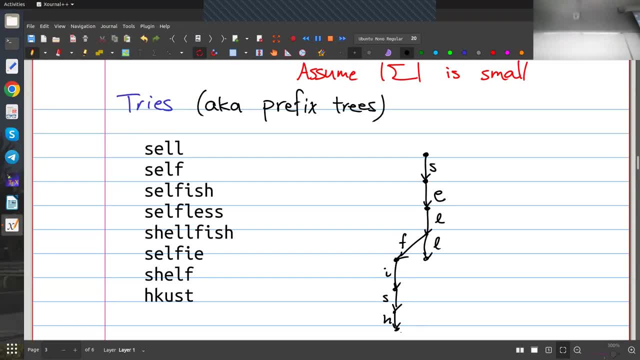 Okay, Now you already see the problem. Just like before, I have to keep track of the ends of my words, Because if I have a try like this, I don't know if the word SELF is in there or not. So I can just have a marker on each one of my vertices. I can just have a checkmark. 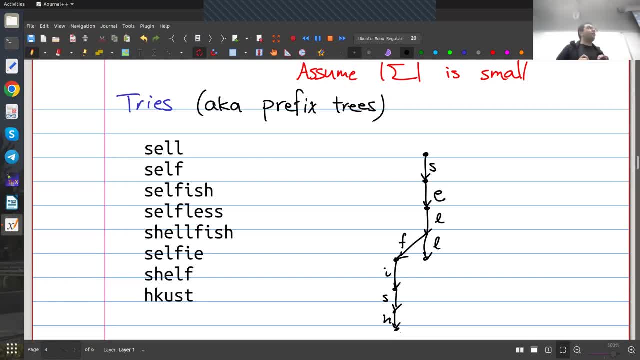 a Boolean flag that tells me whether this vertex is the end of a word. But instead of doing that, I can also do something else. I can just again add one character to my character set And I can say that this is the end of word character. 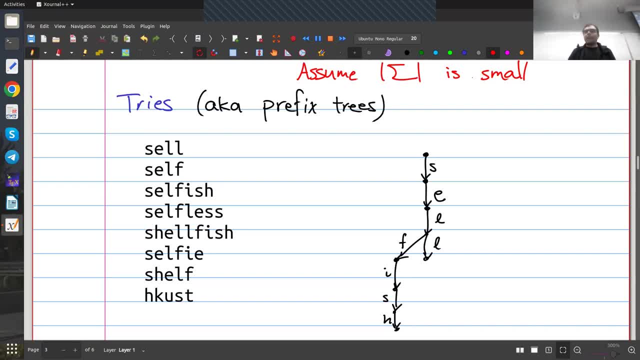 So every word ends in this character And I want my end of word character to be smaller than all of my other characters. So if your characters are in ASCII, I would use something like this: Like a pound hash sharp. I don't know what you call it, But I'll just add this to the end of all of my words: 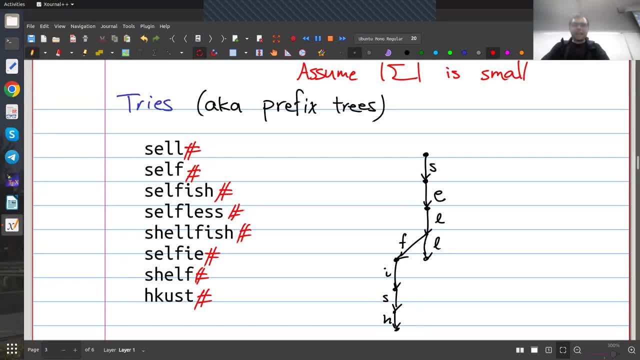 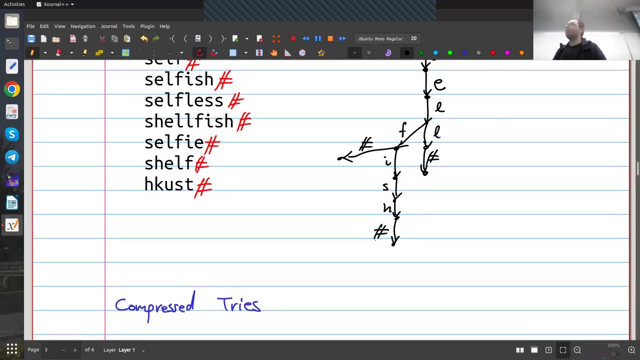 Okay, And now, because every word ends in this character and because this character only appears at the end of the words, I can easily understand which points are the end points of the word. Because now my SEL becomes like this: My SELF will actually have this, And then SELFISH will have another edge with this end of word character. 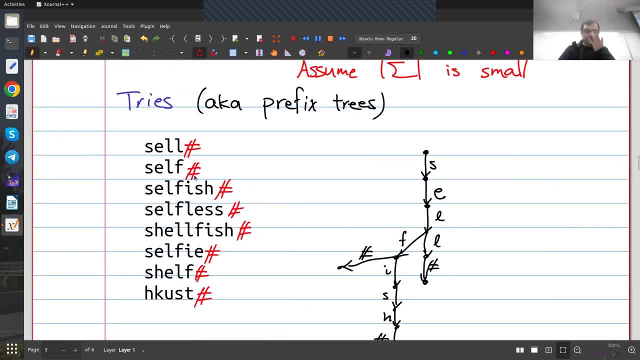 Okay, Now why did I say that the end of word character should be alphabetically smaller than all of my other characters? Well, because, you see, SELF is a prefix of SELFISH And I want SELF to appear before SELFISH. So in order for that to happen, this end character should be smaller than. 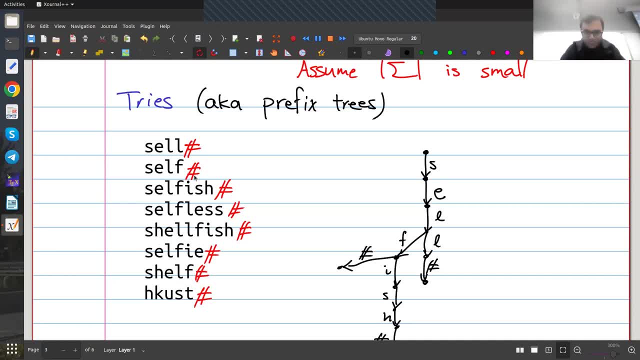 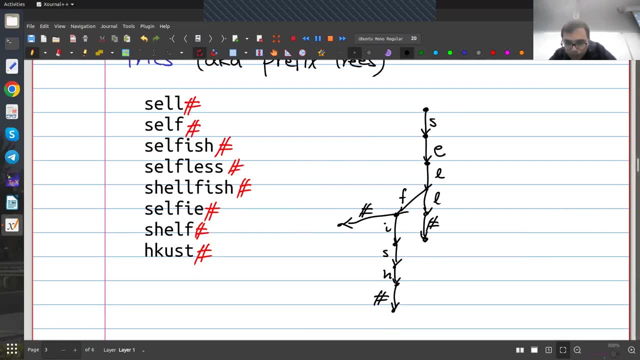 all Right. So that's just a small trick that we play. Now, if I want to add SELFLESS, let's just do this really fast, So I have SELF and then- oh, this is hard to okay. whatever Let's say, I have. 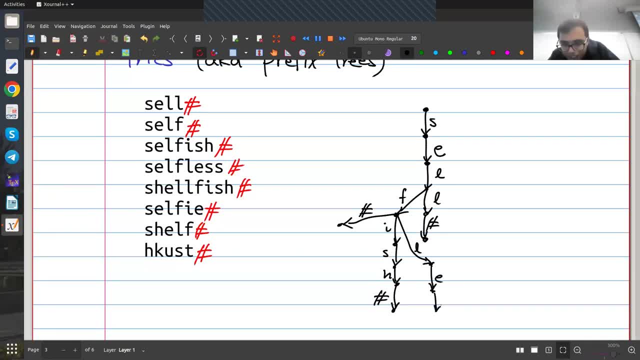 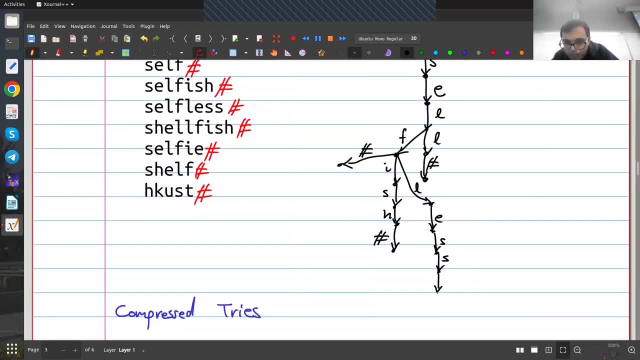 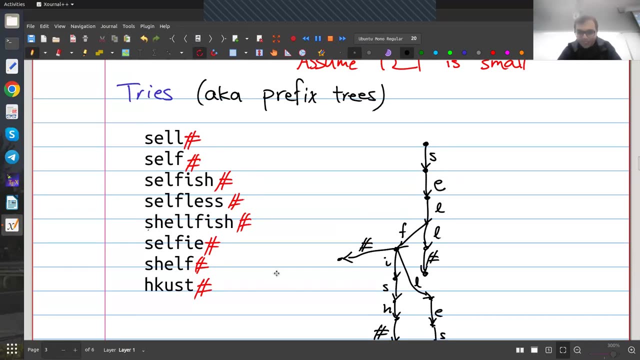 L, E and then S, and then S, And then, of course, I also have this one sharp at the end. Okay, And let's assume that we don't have the rest of these words. I wasn't thinking when I added this example. this would be too large. 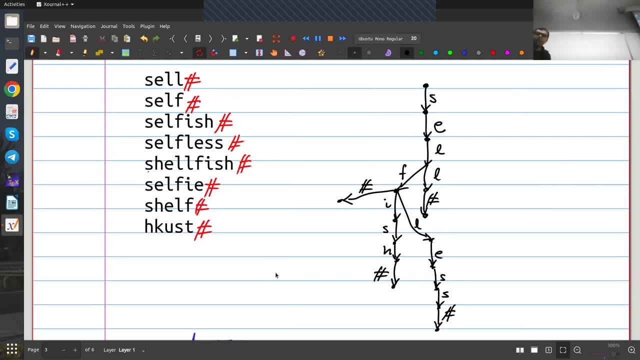 You get the idea. So basically, the idea here is that I'm really saving space, Because whenever two of my words have some shared prefix- for example, SELF is shared between these two words- I'm going to save that only one. I'm not going to save two copies of SELF, Okay. So actually this is going to give me some. 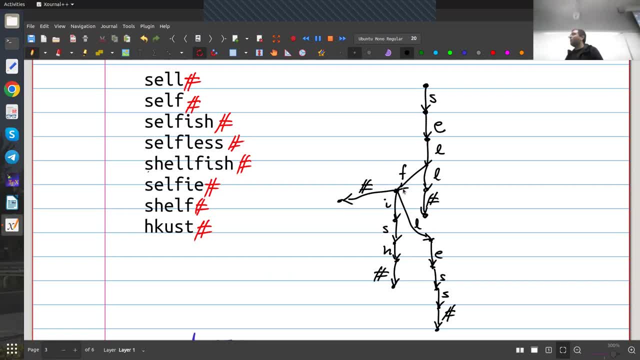 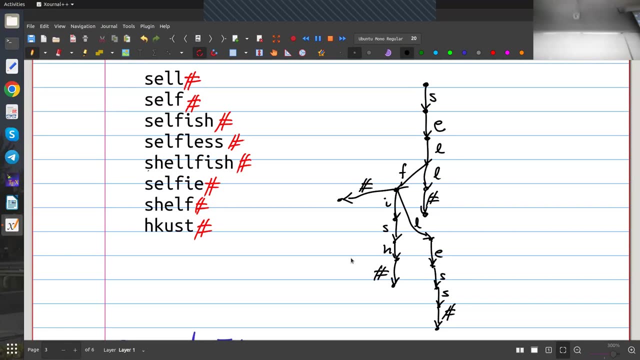 cuts in space. But in the worst case I might have a bunch of words that don't have any common prefixes, and then I have to save everything. But anyway, this is called a try. Now you saw the process of inserting something in the try. You just start at the top, You keep going down one. 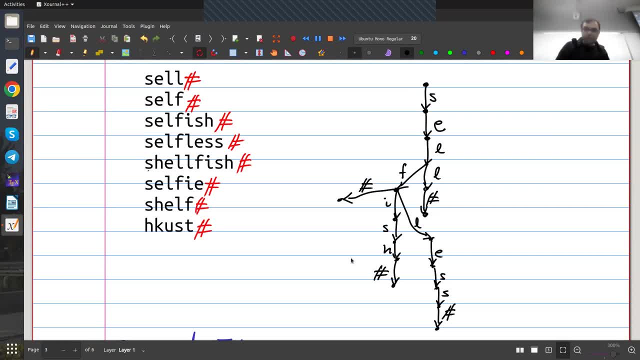 letter at a time And you just start at the top. You keep going down one letter at a time And you insert everything until you get to the end-of-word character. Now if you want to search for something, it's exactly the same process. I just start at the top. So let's say I'm searching for 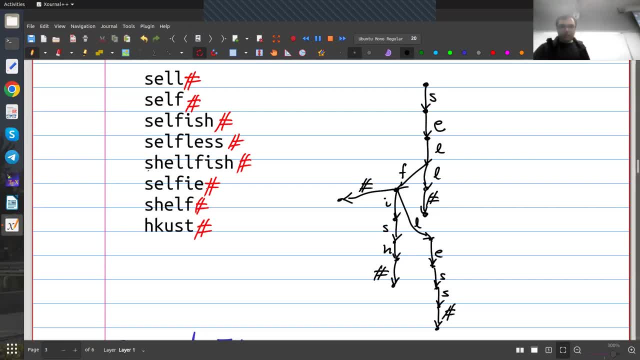 whatever SELFY. So let's say, I'm searching for SELFY and I haven't inserted SELFY yet. So I start here. I take the first letter, which is S, and then E, and then L, And then here I know that. I have to take F, And then I have to take SEL4.. And this is interesting: I take the first letter, which is S, and then E, and then L, And then here I know that I have to take F, And then I have to trek. 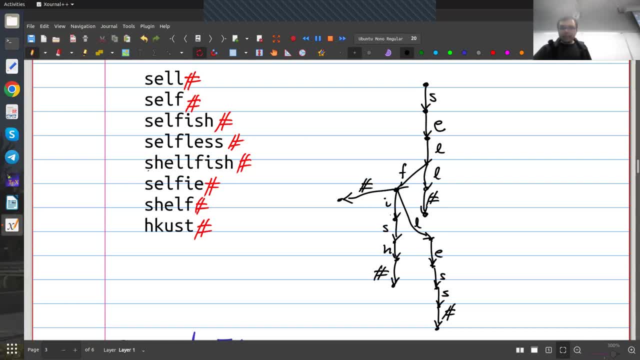 SEL to 5. And then I have to take M, and then I have to take space And finally SE and then fire. See if we can do that. i- and at this point i'm looking for an e, but this vertex does not have a child that is labeled e. 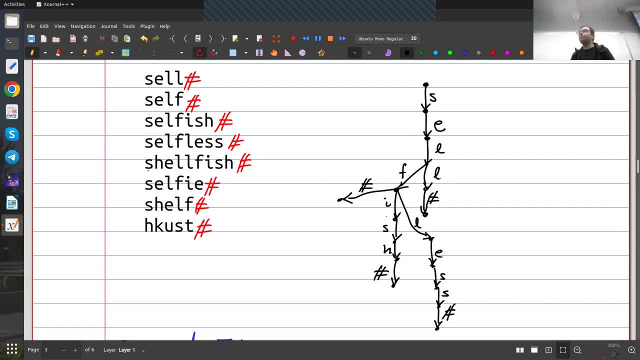 so that tells me that the word selfie is not here. okay, and again, remember that when i'm searching, i also add this end of word character to the end. so if i search, for example, for the word just s, e, i would start here s and then e. i could take all the edges that i was looking. 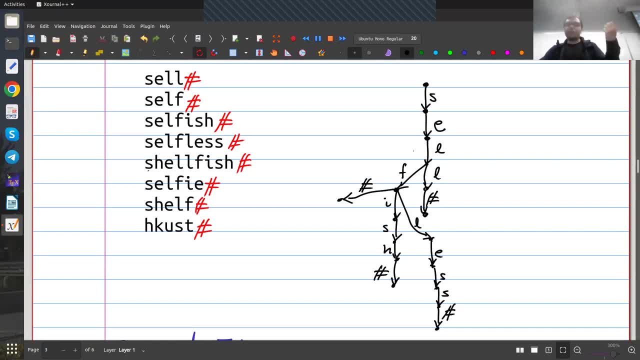 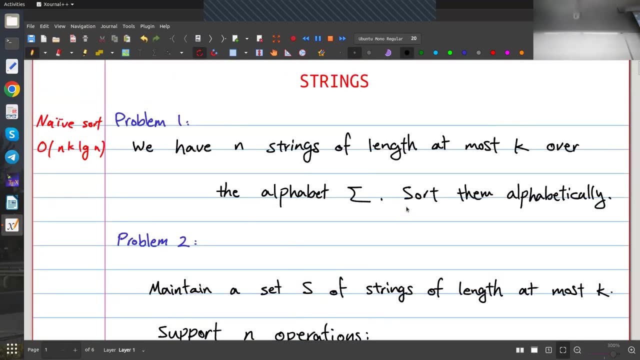 for. but then, remember, i have an end of character, end of word character as well. so here i'm looking for the end of word character and that doesn't exist. so i say that this word was not in this set. okay, going back to my problems, let's see i have n strings of lengths, at most k, over this alphabet. 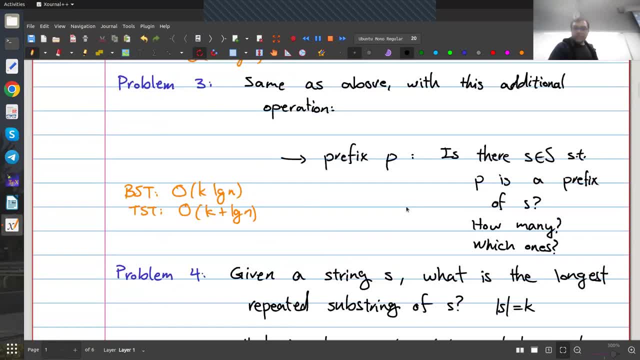 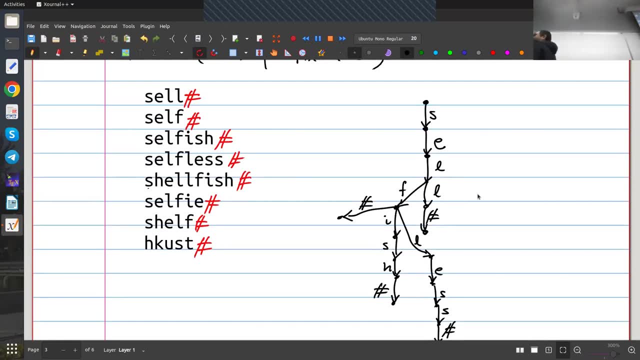 i want to sort them alphabetically. well, let's add all of them to a try and then, when i have this try, i can print everything alphabetically. right, just start at the top and every time take the leaf that has the smallest label, right, that would give you the first word alphabetically and then continue. 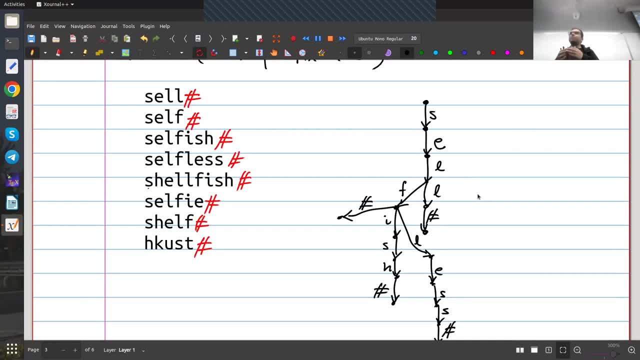 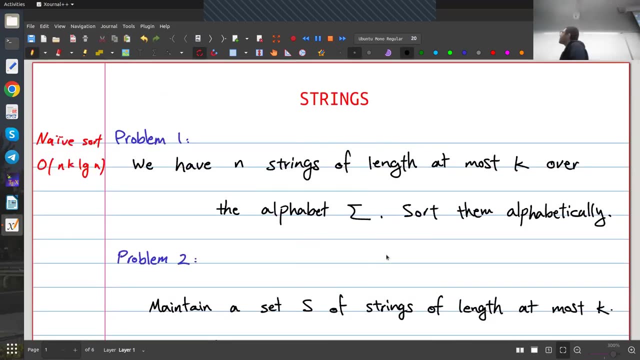 doing that. basically, it's an in order traversal, except that i just assume that the leaves are in alphabetical inside. the children of every node are in alphabetical order. okay, but how much time would this take? well, i have to basically add n streams, but when i'm adding a string of lengths, k. 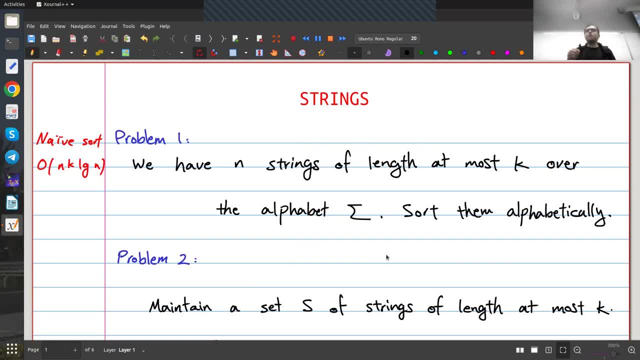 that's taking only o k time because i'm spending constant time for every character. i'm starting at my root for every character. i'm spending only constant time to either create the node that i didn't have or go to it. if that node existed, okay, so creating it would take onk, and actually then going over it and printing all of them. 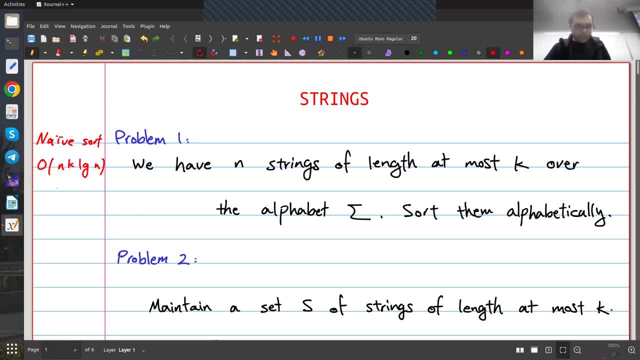 would also take onk. you can't tell if it's gonna take long or connected to its last space, okay. okay, Fantasy Seeds and you'll have to think about all the weievous guys front to back like by. the can just analyze that later because we're running out of time. so this is onk, if i use a try. 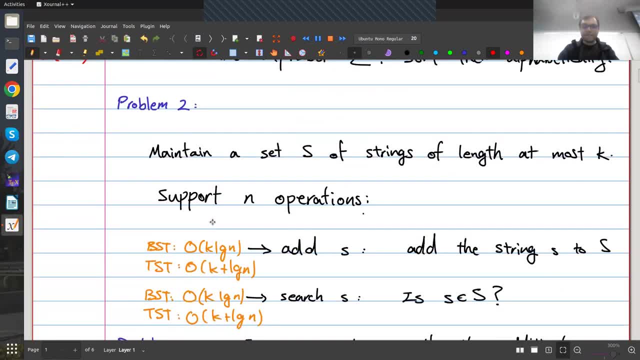 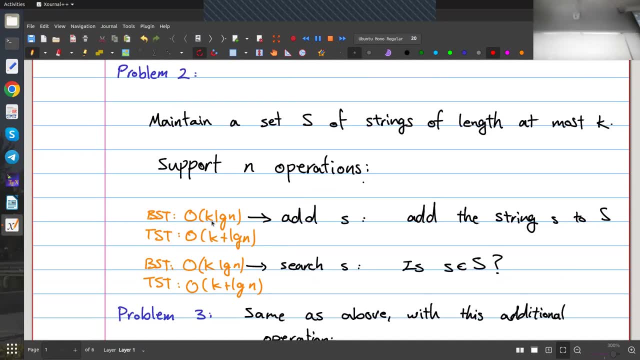 what about these operations? so again we have adding and searching. we saw both of them already. adding a string takes okay time and the fun point here is that this is independent of the number of strings that we have. so my n is not even appearing in my runtime, but of course i'm assuming that my 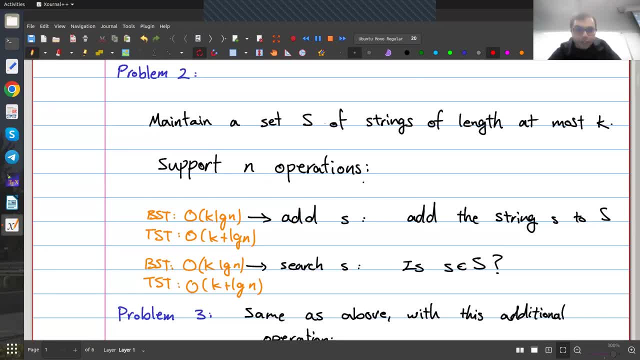 alphabet is small, right? so in a try, adding a string is going to take okay time, and then searching for a string is also going to take okay time, which is now better than all of the solutions we've had until this point, because of course, it's better than k plus log n okay. 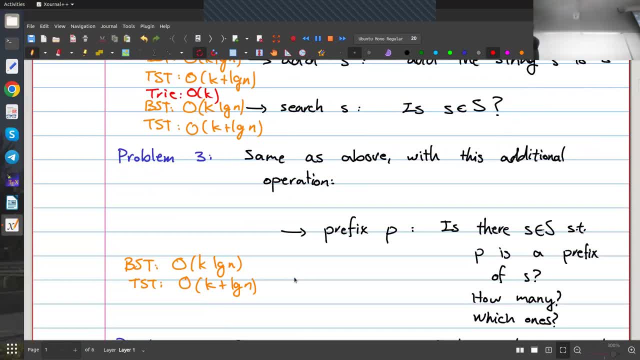 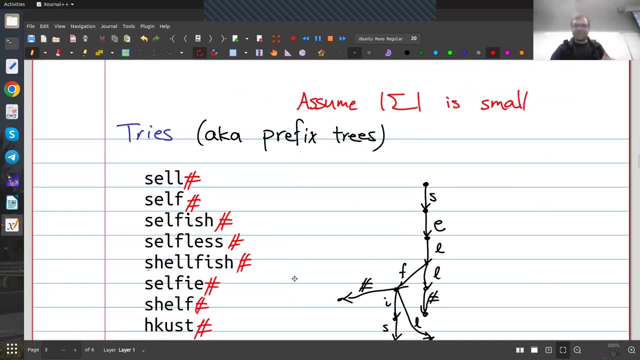 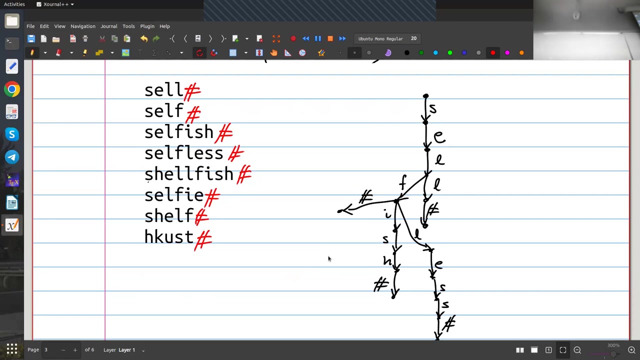 what about this one? i'm given some string p and the question is: do i have a string s in my set such that p is a prefix of s? well, the nice point about a prefix tree or a try, is that basically every note here corresponds to a prefix of one of my streams, right? so, for example, if you look at the string 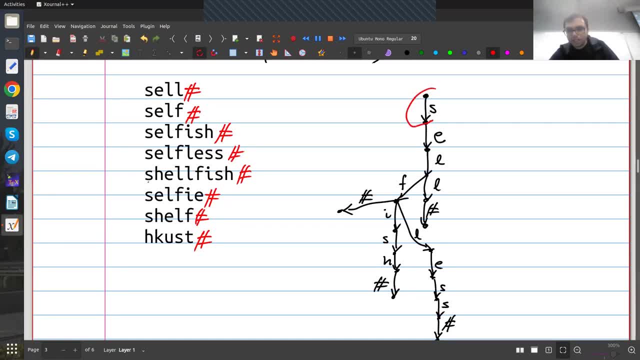 string n. the string n is going to be a prefix of one of my strings, right? so, for example, if you look at the string string p is going to be a prefix of one of my strings, right? so, for example, if you selfish, this is one prefix of selfish, just s, which is this node. this node corresponds to se. 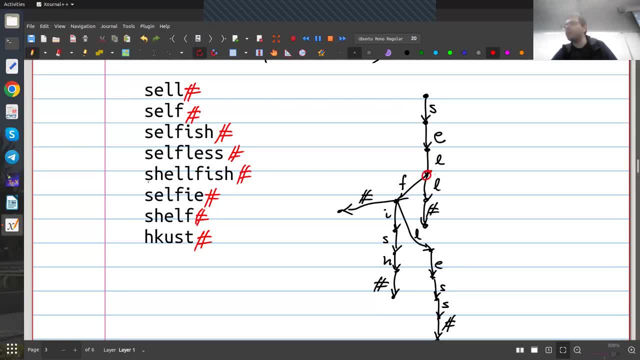 which is the second prefix. this node corresponds to sel, which is the third prefix, and so on. so every prefix corresponds to one node and every node corresponds to one prefix. so if someone asks me, for example, is there a word here that has sel as a prefix? i just search for sel. 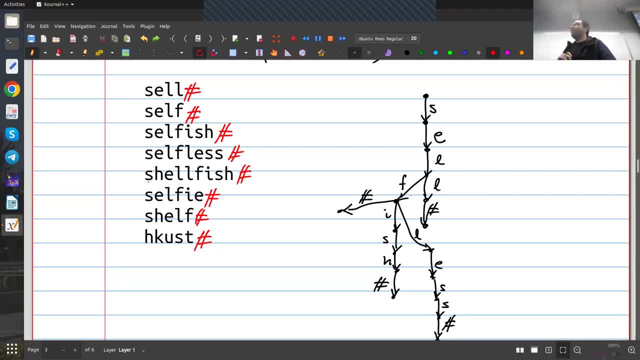 i just don't add the end of word character at the end of it, and when i find sel, i say yes, i can also count right. so here's the thing: when i'm inserting at every node, i can also have a counter which basically tells me how many times did i insert something at this node and its. 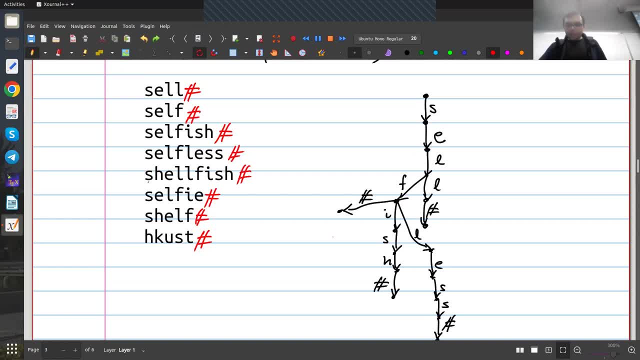 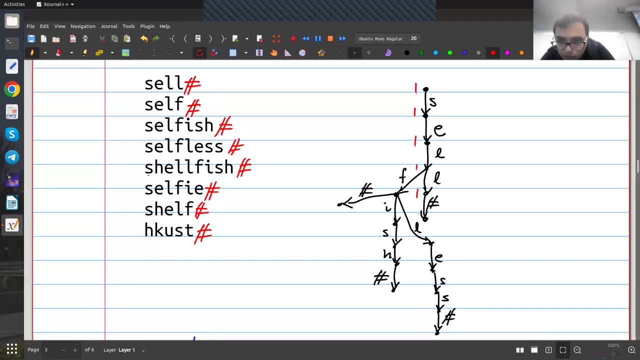 descendants right and then. so, for example, when i'm adding sel, i would have my counters like this: one, one, one, one, one one. And then when I add selfish, all of these increase, they become two, two, two, two. 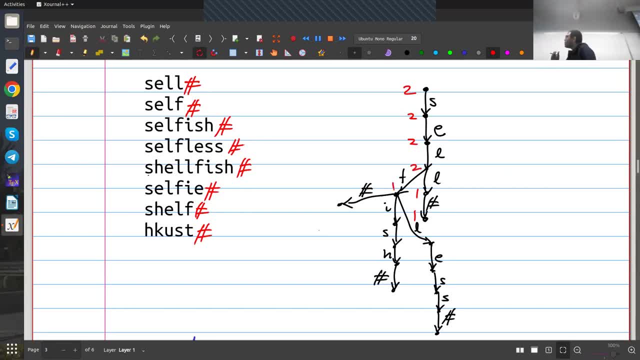 but then this F becomes one, and so on. So every time that I'm adding something, I can just keep a counter at each one of my vertices- Remember how many times I've seen them when I was adding strings. And then, if I look at the counter at S E, 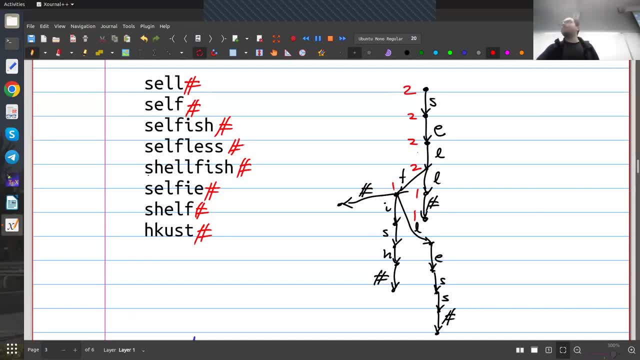 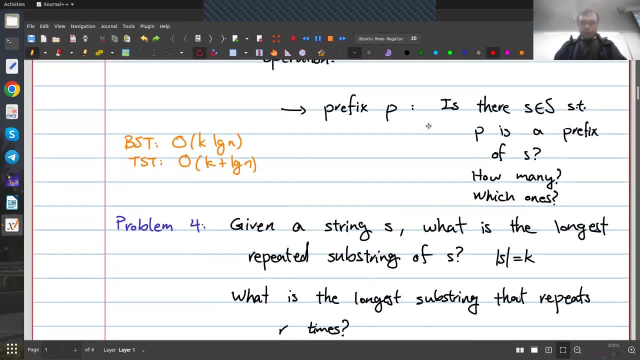 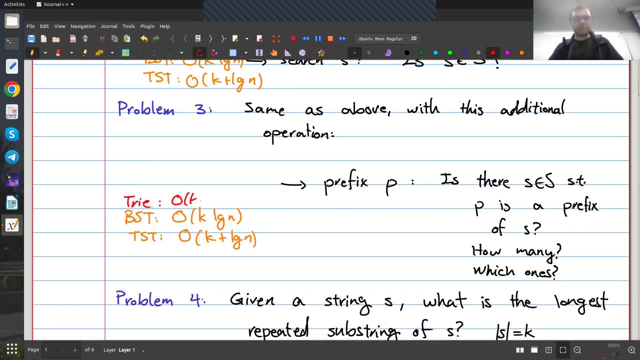 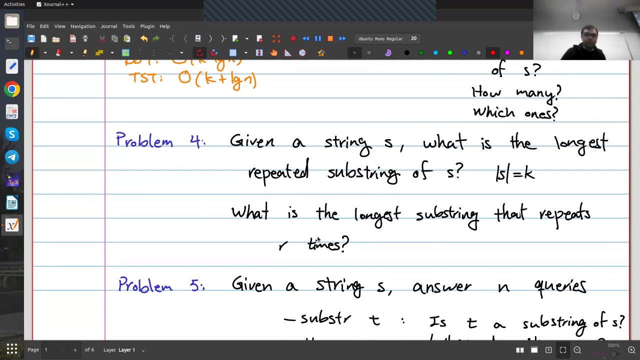 that would tell me how many strings have S, E as a prefix. So, again, this also solves this problem in: okay, What is the longest repeated substring, and so on. We're not going to have better algorithms for this at this moment, but we'll continue on this. 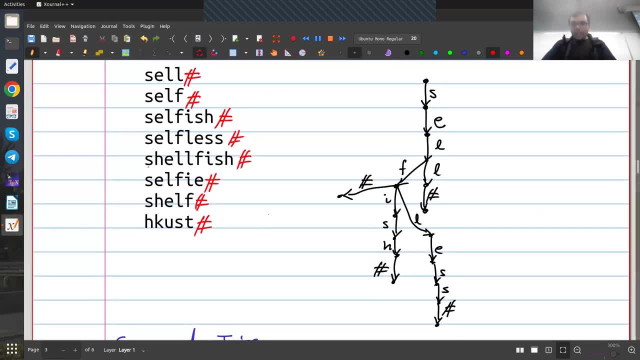 Okay now, one problem you might see here is that pretty much wasting a lot of space, And so my runtime is kind of optimal, because whenever I was reading some word I had to at least spend some time proportional to the length of the word, because I have to read it. 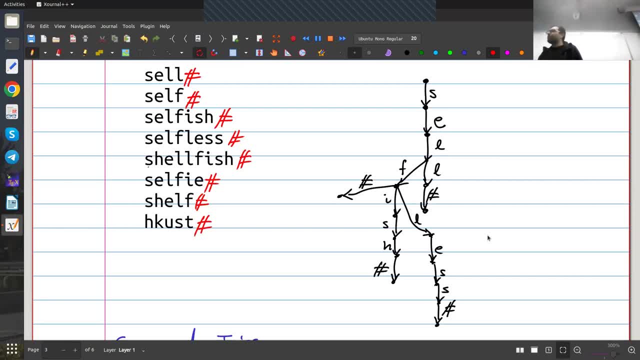 And I'm spending just that amount of time to also save it. So my runtime is fine, but what about my space? I'm using a lot of space here. Could I use less space than this? Well, actually not really if you're talking asymptotically, but I can reduce. 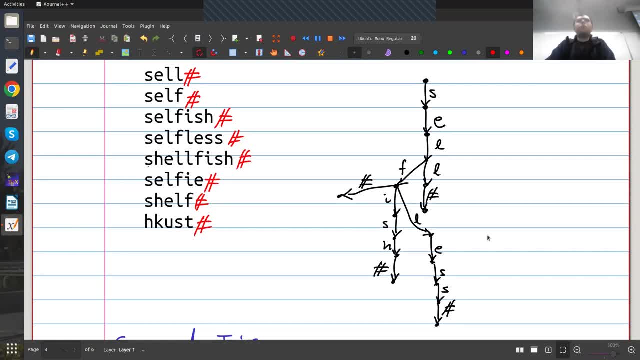 the number of nodes that I have in my tree. So, how many nodes do I have in this tree? in the worst case, My worst case, would be if none of my words, uh, share any prefix at all, And if they don't share any prefix, then I would just have one vertex for every. 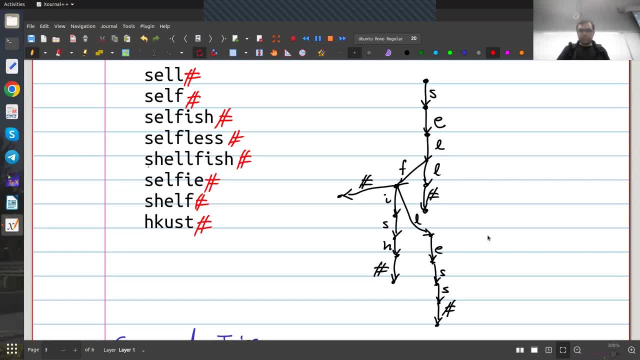 letter, I would have O and K uh vertices here now. can that happen if I have only a limited alphabet? so let's say, if my strings were only over zero and one, would it be possible that I still have Uh, a huge try. 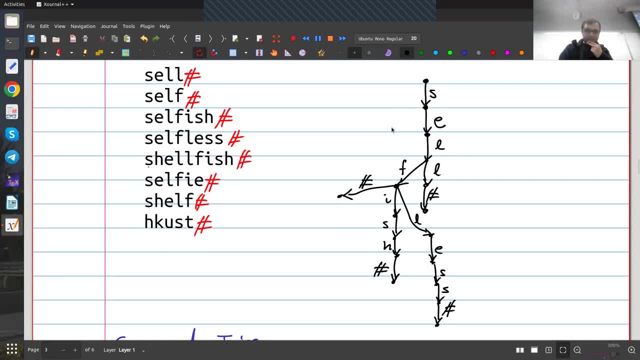 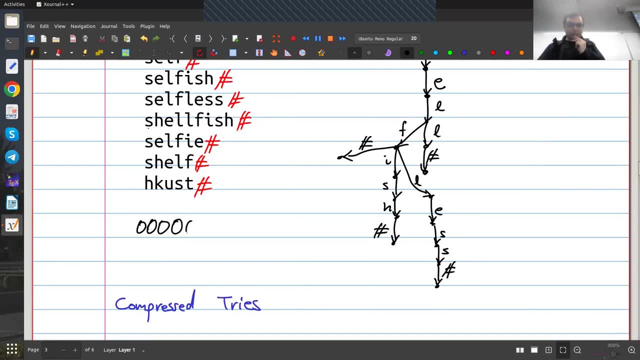 Yes, actually that's can happen. uh, because I can have something like this: Let's say, I have a bunch of zeros followed by a bunch of ones, and then I have one fewer zero followed by the same number of ones, and then something like: 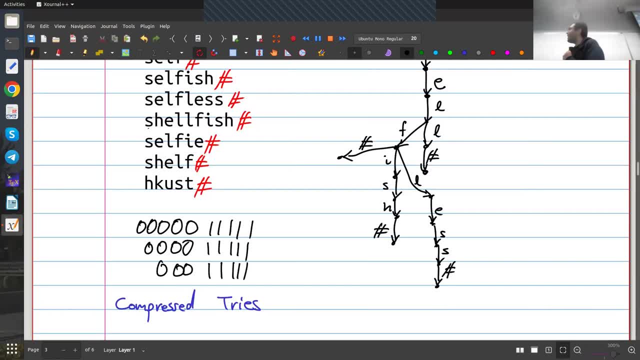 this with the same number of ones and so on. And If you See this, if you put this in a try, you will of course have all of the zeros, but then, branching out of each one of the zeros, you will have a lot of ones. 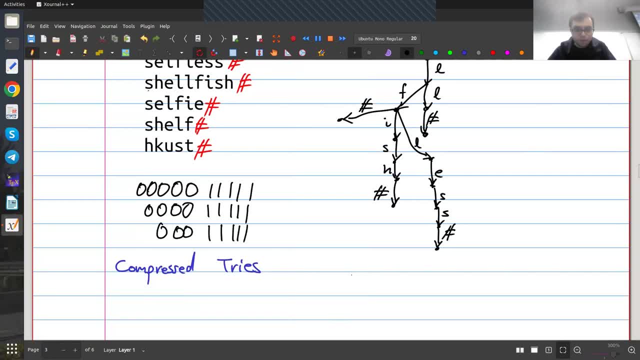 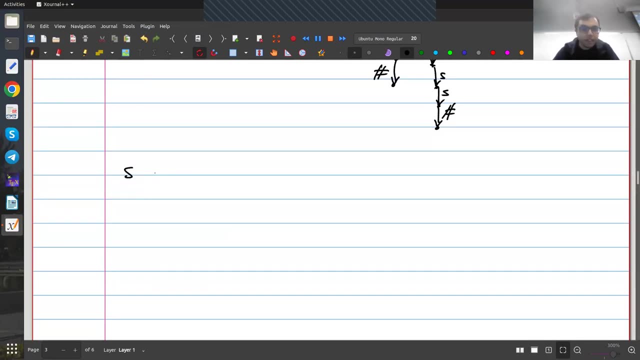 Okay, So let me show this to you. So this is what I want to say. I want to say I have a bunch of strings and let's say that my first string has a lot of zero. So let's say K zeros, followed by K ones. 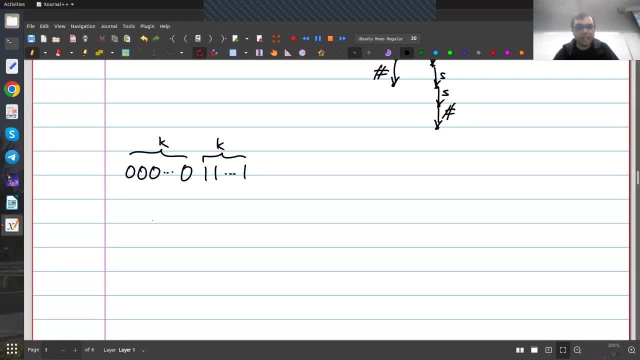 Okay, My second string has K minus one zeros followed by K ones, And then the next one has K minus two zeros followed by K ones, And so on, If I create a try out of this. So for the first one I 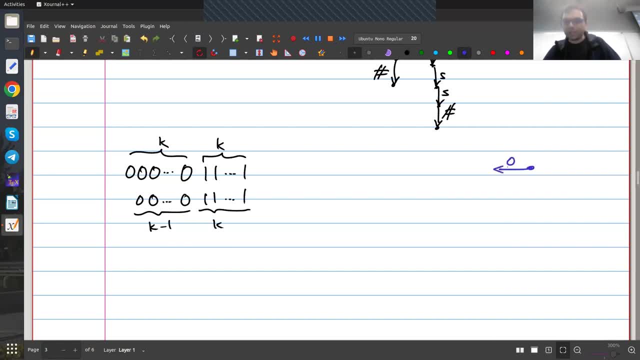 Will have. I'm going to draw my try in a weird way because I want it to fit, So I will have a bunch of zeros. This is my roots. Okay, I will have a bunch of zeros, So there are K of these. and then I have the ones, and there are K of these, right? 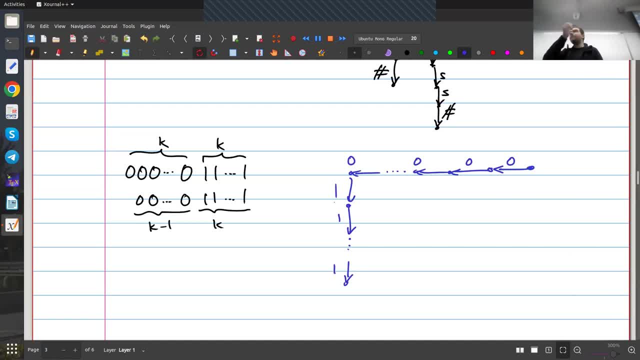 But then in my second string I have K minus one zeros And then K ones. So it starts from here and gets all of these ones, And then in the next one I have K minus two, and so on. So, as you see, I will have a whole grid, basically here. 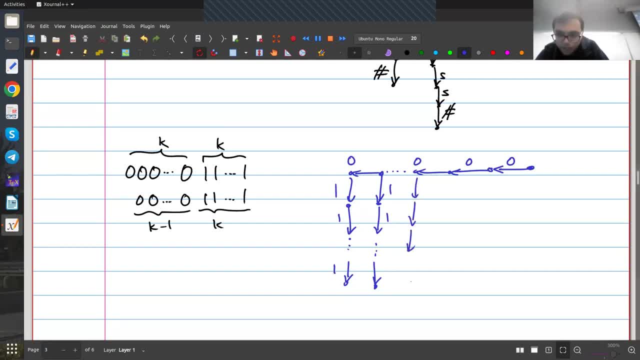 So I will have all of these edges as well in my try. And this is bad because this is K by K. It's like a K squared, Okay, Okay. So yeah, The fact that common prefixes are saved only once can actually save us a lot in space. 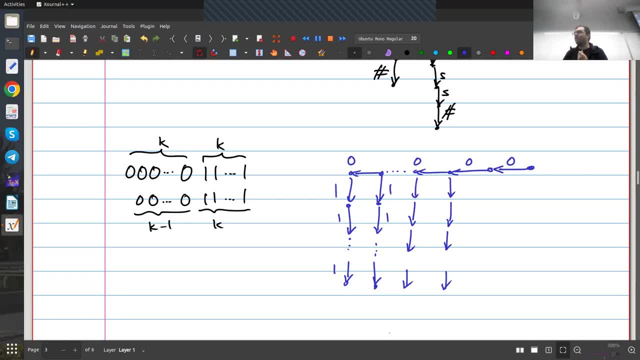 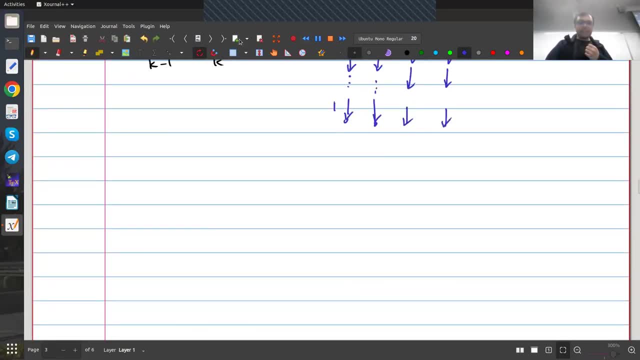 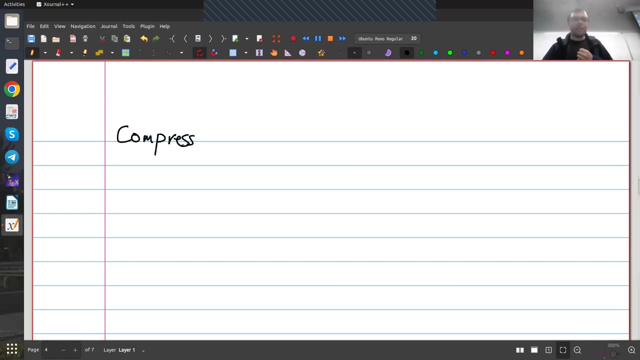 But in the worst case it will save us almost nothing, or just the constant factor. Okay, But uh, we have this thing called a compressed try, and let's see what a compressed try does. So the idea in a compressed try is that I want to have a try, but I want to have fewer vertices. 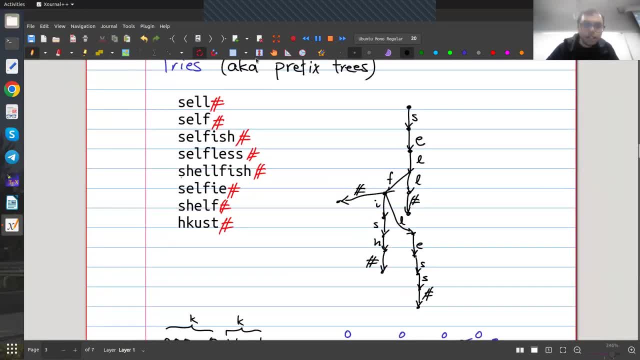 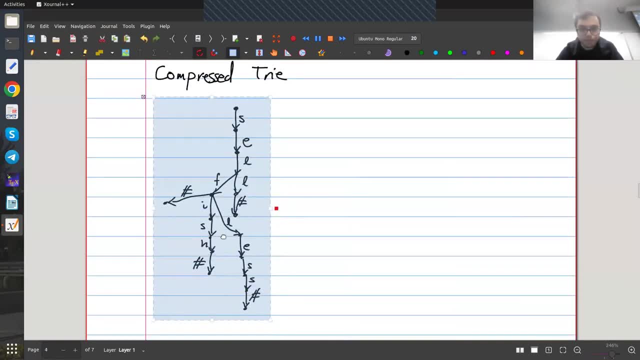 So let me just copy my try from here. This one really looks ugly. This is my try. Now, if you look here, there are a lot of vertices that have only one child, So there is no reason for them to be vertices at all. 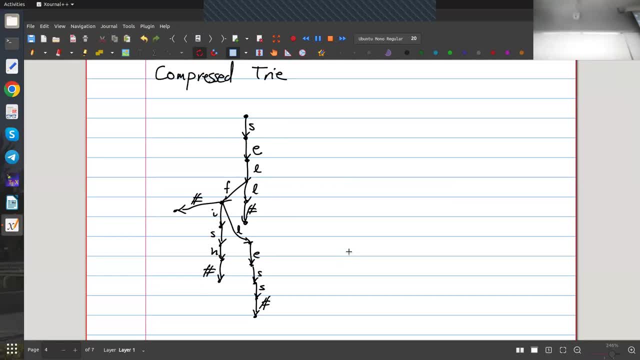 Right. So, for example, I have this whole path here, S E L. I could just have one edge Instead Of this whole path. So I could create something like this: I could say: I take this S E L and I just merged it into one edge. 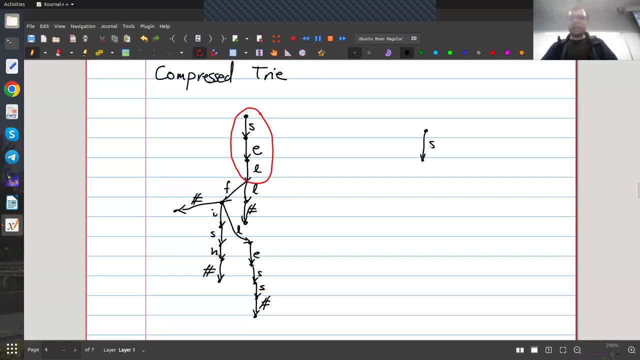 So I will have one edge. And now the label of my edge is not just one letter, It's the whole string. It's S, E, L, Right, And then it has two children. One side is F, On this side I have L, sharp, but again I can just merge these two. 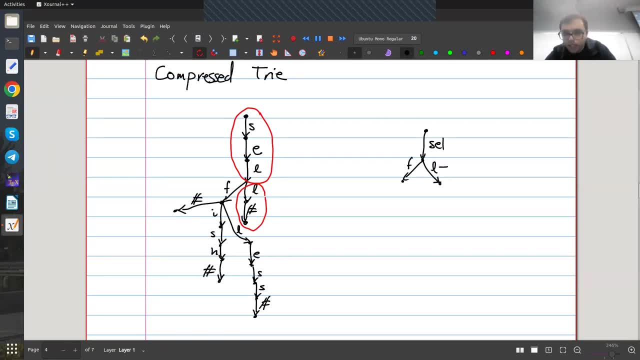 So I can just have one note here and I can write L sharp on this edge. Now I can do the same thing for F, so I can merge all of these. I can merge all of these And of course this one is merged already. 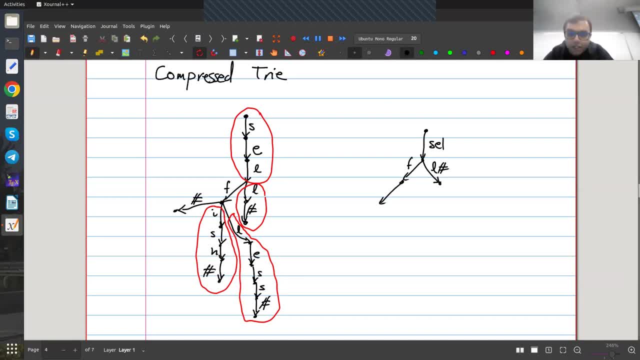 So F can have a child here That is just sharp. It can have another child And this child is a ish sharp, and then it can have another child Which is labeled less sharp. Okay, So I could compress my try to look like this: 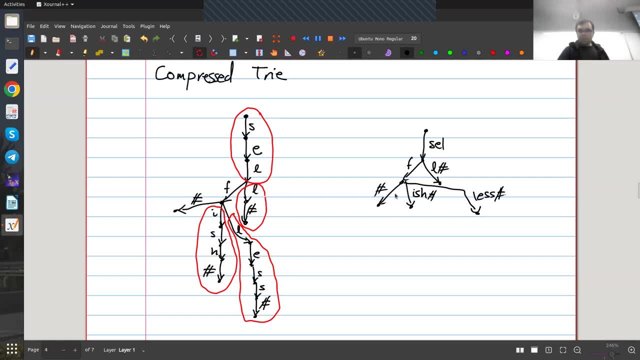 The only difference is that now, uh, when I'm traversing an edge, I'm basically traversing several letters at the same time. Now, does this help? Does this actually take asymptotically less memory? No, Why? Because, even though I have fewer vertices, I'm now saving these labels, which are much longer. 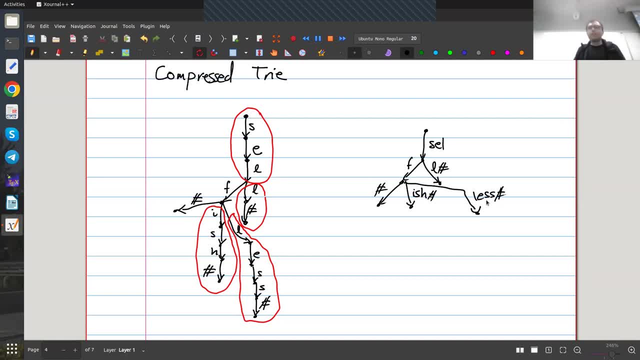 So if I'm saving a label of lengths K, that's taking K units of memory. So in terms of saving memory, I mean it's. I mean I have fewer nodes, so maybe I'm reducing my memory by a constant factor, but it's not going to make a big difference. 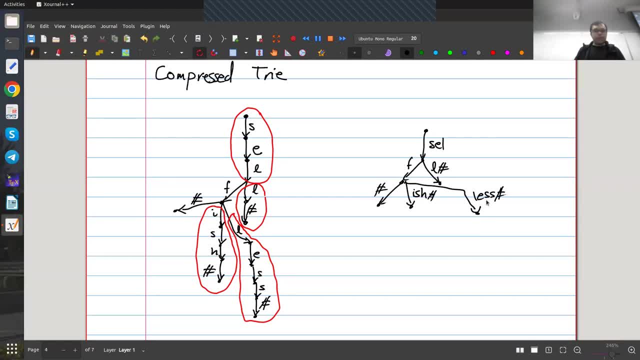 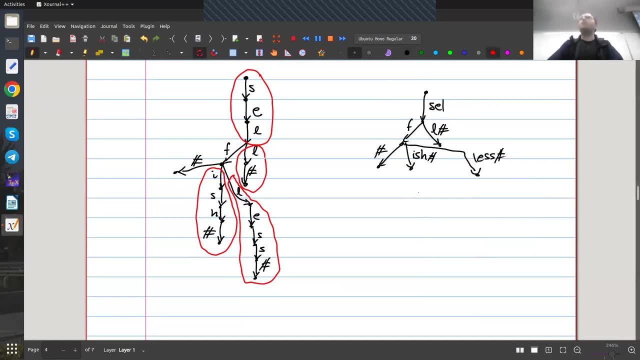 But what about in terms of saving notes? actually, how many notes can I have? So here's the thing. Let's just uh forget that N and K were different And let's say I have N strings of lengths, at most N. 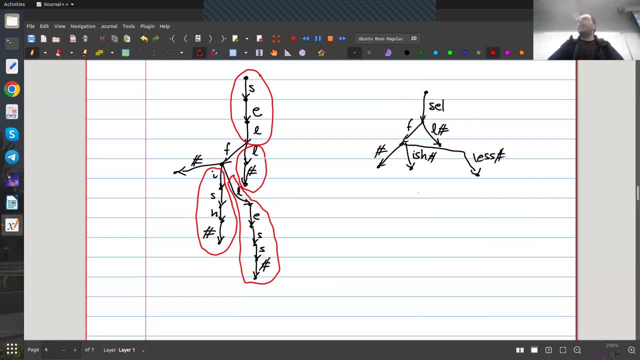 So I'm going to use N both for the maximum lengths of my string and also for the number of strings. So here It was possible that I had N squared notes, even if my alphabet was very small right, Or in general I could have NK notes. 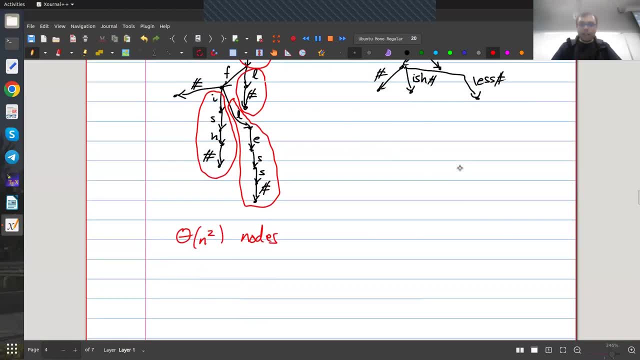 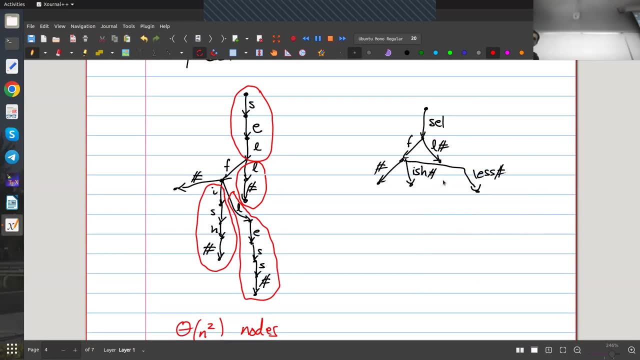 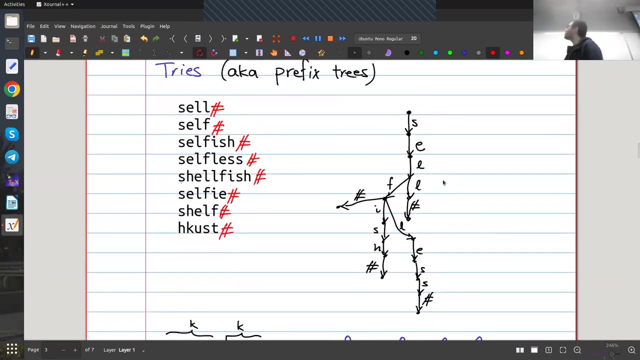 And that's the example that we had here, The example of the grids. but how many notes can I have in a compressed Right? So, in order to answer that, I have to go back to my Try and I have to show you something else, because I added this short character at the end. 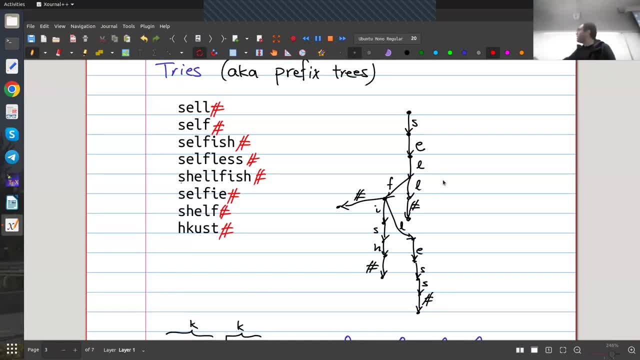 Every one of my words is now saved at a leaf of this Try Right. And also every lead corresponds to exactly one word, because all the leaves have an edge with sharp going into them. So all the leads are at the end, Okay. 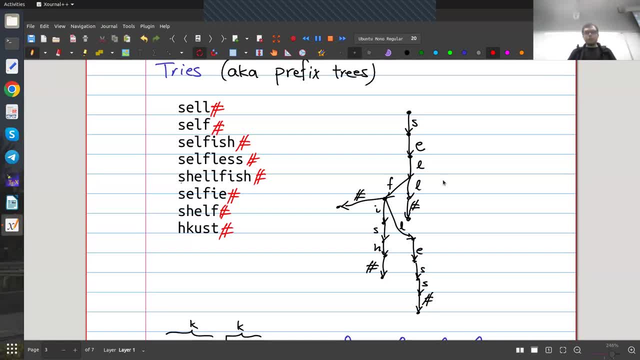 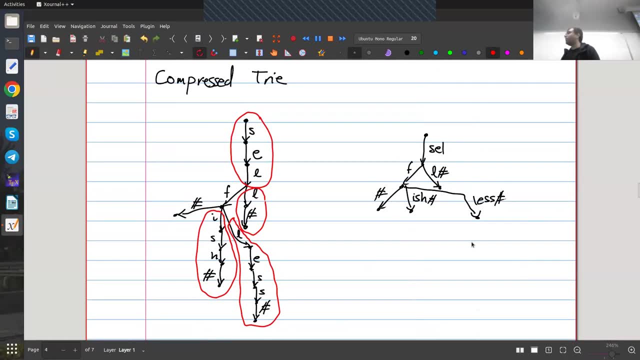 So My number of leaves is exactly equal to the number of words. Now, when I do this compression, I'm not changing the number of leaves. I can again do the same argument. I can say: every leaf has a label that ends with a sharp, instead of just being exactly a sharp right. 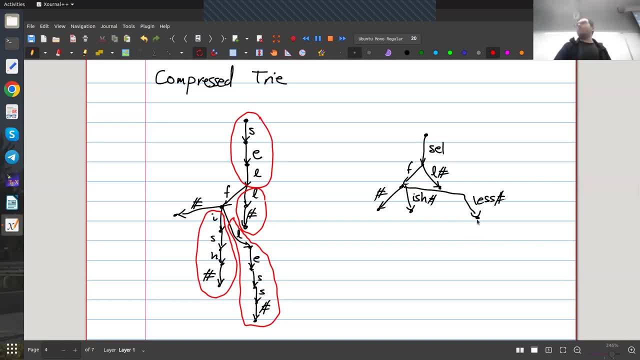 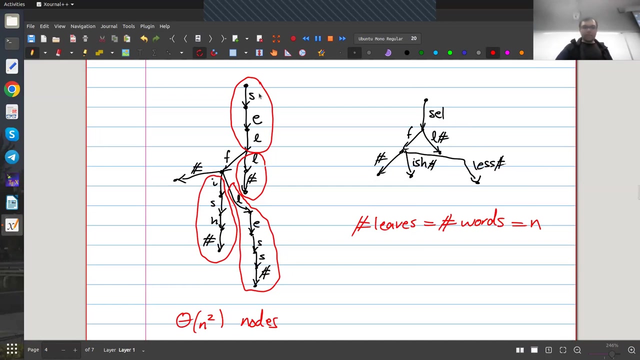 And, uh, every label that ends with a sharp is also a leaf, and so on. So, Uh, the number of leaves is basically the same as the number of words, which we said is okay, great, But now in the normal, try, if I had a bound on the number of leaves, it wouldn't give me a bound on the number of notes, because I could have things like this: 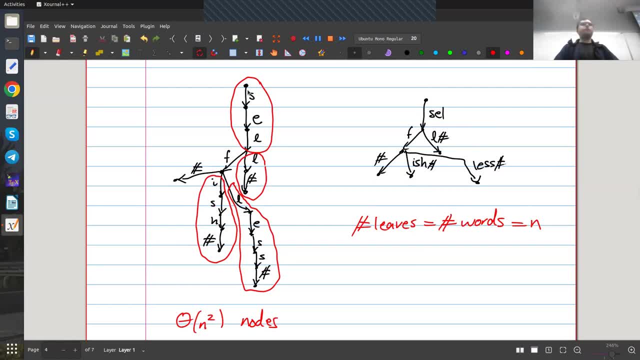 This is like I could have a huge path. This is like I could have a huge path That contributes only one leaf, but here every note that is not a leaf has at least two children, because if it had less than two children, I would just merge it up. 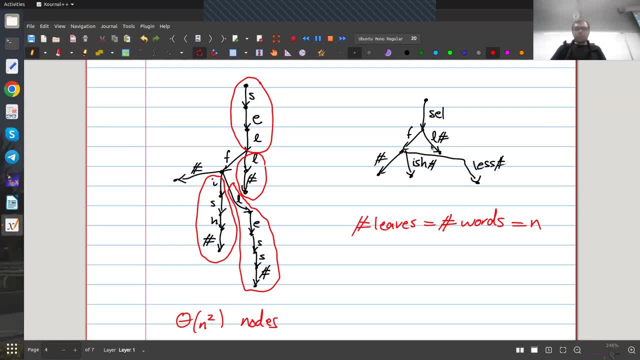 Right, So this is a binary tree. It's not a complete binary tree, but okay, No, not binary, It's at least binary tree in the sense that every more than binary, I don't know. Okay, Okay, Okay. 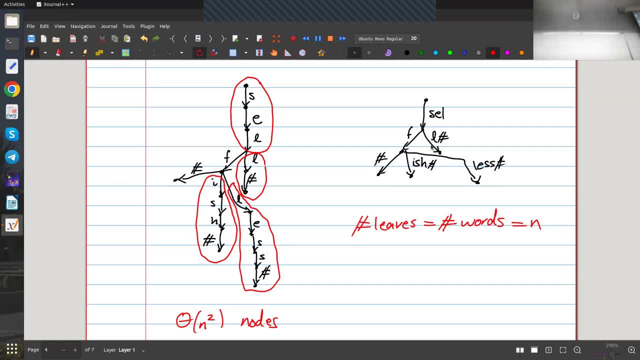 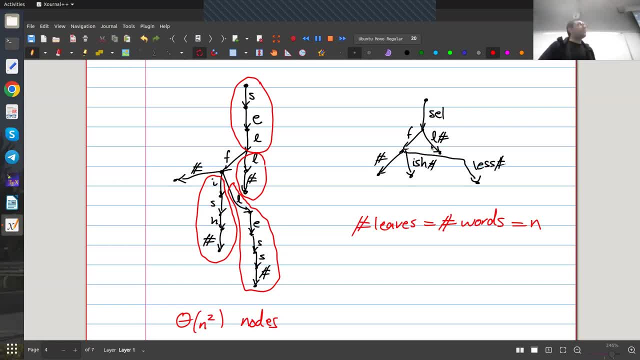 Okay. So what is the number of non-leaf notes? It's, at most, N. Now why is that? Just look at it as a DSU problem. for a second, Suppose that I have a DSU on my leaves. Initially, all of my leaves are in different sets and then this note is like a merge operation. that is merging. 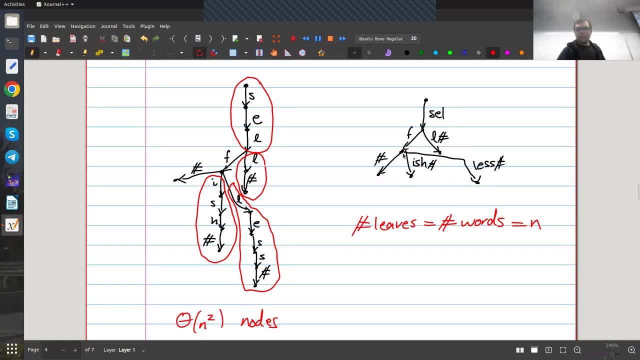 This, This note, is like a merge operation, that is, merging this one and this one and so on, Exactly like a DSU data structure, right? So if I start with N different sets, how many times can I merge? I can merge at most N minus one times, right? 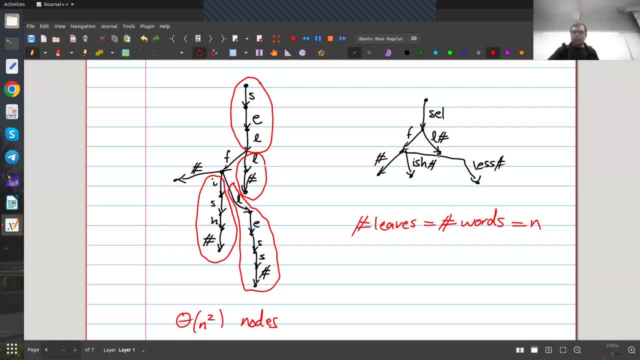 And eventually I will just have one set. So, and every merge corresponds to one of these internal nodes or the non-leaf. So the number of non-leaves, Okay, Is also in O of N, It's at most N minus one, but I only care that it's in O of N. 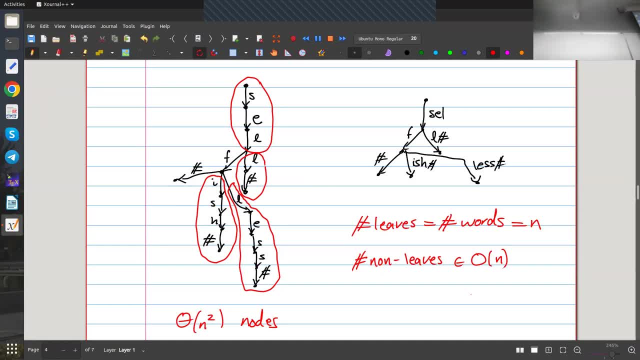 So the total number of nodes in a compressed dry is O N. Now this doesn't really make me happy because even though the number of nodes is small, because the labels are long, I have to potentially save a label of length K at each one of the edges. 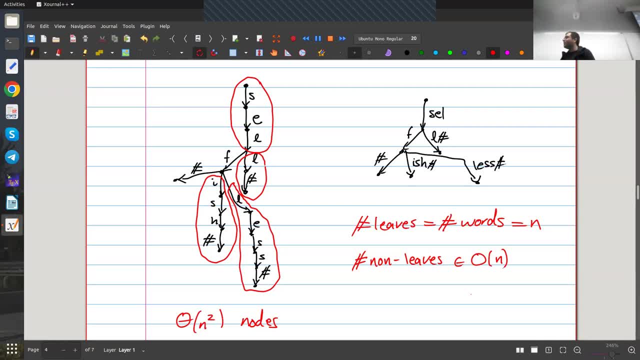 So it's still going. It's going to take O and K, It's going to take O and K space, And I mean you can also create it in O and K time. You can create this by either first creating the uncompressed version and doing the compression. 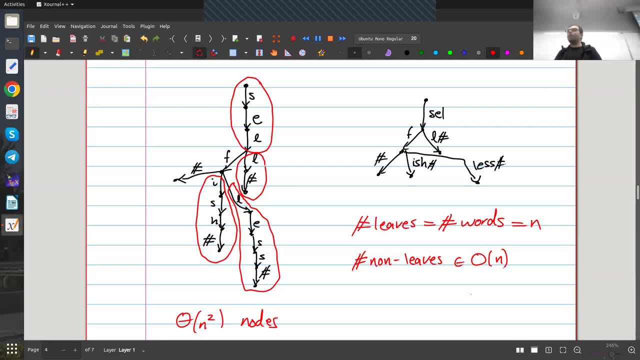 or you can just do your insertions on the compressed version. It's very similar. You have to just be careful. Sometimes you're traversing like half of the label on some edge and then you have to cut that edge into. Okay. 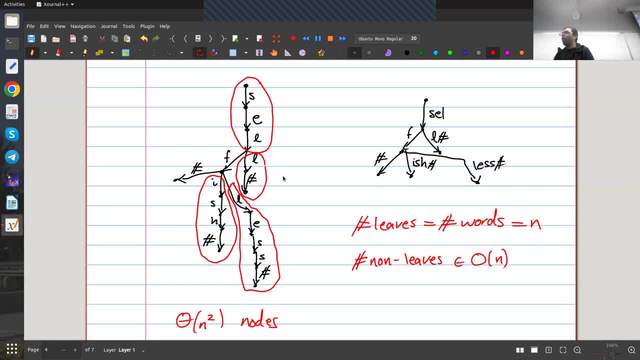 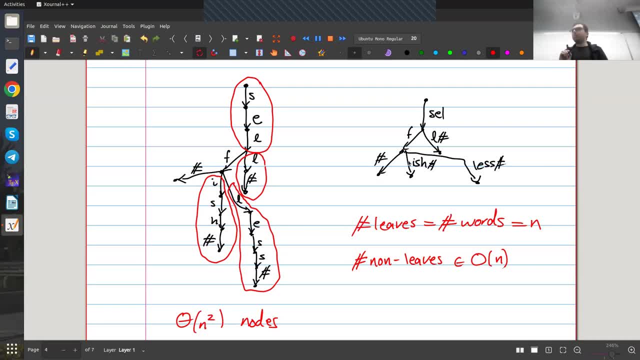 but unfortunately it's still taking a long time to create and it's using a lot of space. Now, in the next session, we will see that this is actually useful, because in some cases I don't have to save the labels, And in the next session we will see that when I don't have to save the labels, when 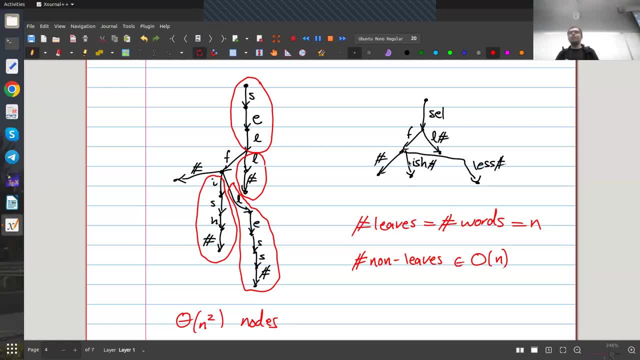 I can just have, let's say, a pointer instead of each one of the labels, then the label will run automatically. this is great, because this is giving me all of these operations and I could create it in O and then I can query the existence of a string in okay, and I can. 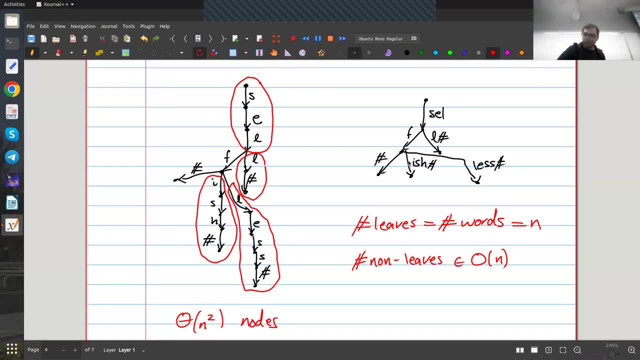 add new strings also in. okay. okay, I'll see you tomorrow.